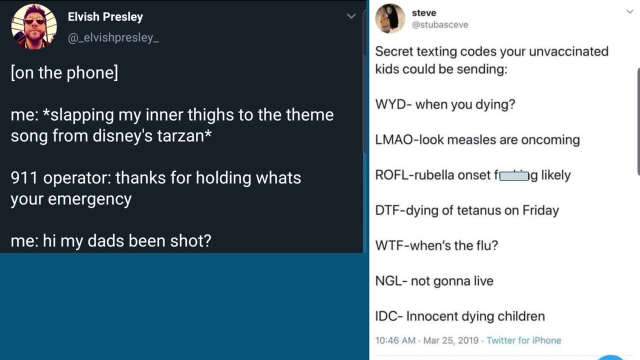 You have to know that for, like, I want to say like ten different species, right, And I see students make the mistake of saying I'll memorize it like a few days before the test So that it's fresh, right, It's a lot of stuff And it's pretty not like vague, but it's kind of random, right, Like there's not really a great way to remember that Australopithecus was from like three million years ago and Lucy was the famous you know, like there's not really a good way to do that. So start now, right, Don't get comfortable, especially because exam two is in, like. 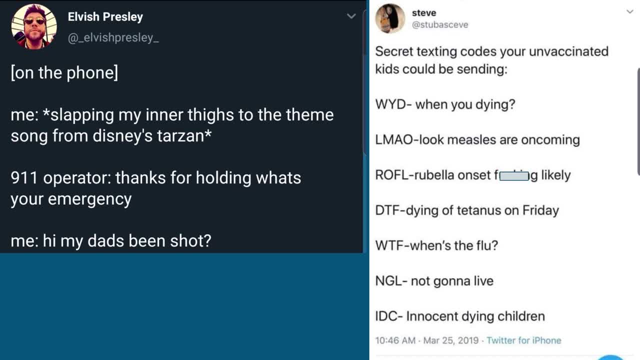 a week and a half Exam four. right, I say exam two. It's in like a week and a half, right? I think so. So it's going to come up very fast. Just start working on it now. That's essentially what this whole rant is about. 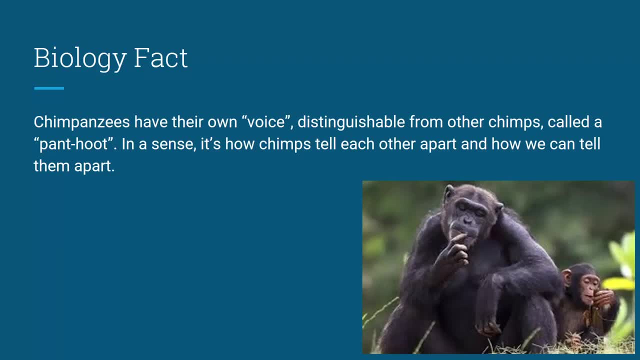 So paleobiology and then human evolution, Your biology. fact for the day is that chimpanzees actually have their own voice that we can tell apart from other chimpanzees, called a panoply, And the way that they make this noise is completely distinct from every other chimp, at least within their social group. So it almost functions as like their name. You know what I mean. It's not like that's what they call each other, but that sets each chimp apart from each other. 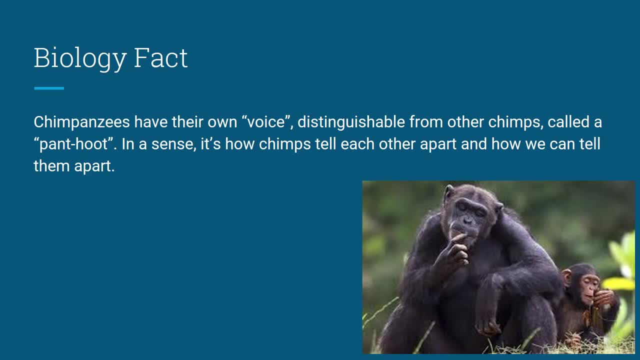 So they actually do have an individual identity And humans actually can even tell the difference between their calls. So humans- obviously you have to spend some time with them, But you know their caretakers and stuff like that- can recognize each individual chimp. 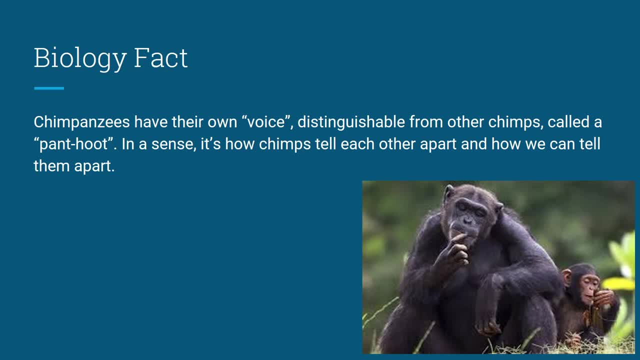 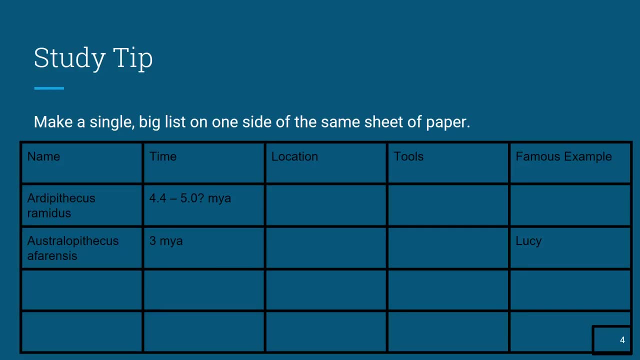 Not just based on their physical traits but on how they sound. So I thought that was kind of wild. They'd never heard of that before. So the study tip goes along with what I was kind of already saying: Make a chart or a graph or some kind of something. This is what I did, And I didn't fill the whole thing out because I didn't want to take the time to fill the whole thing out. It's just to show you right. 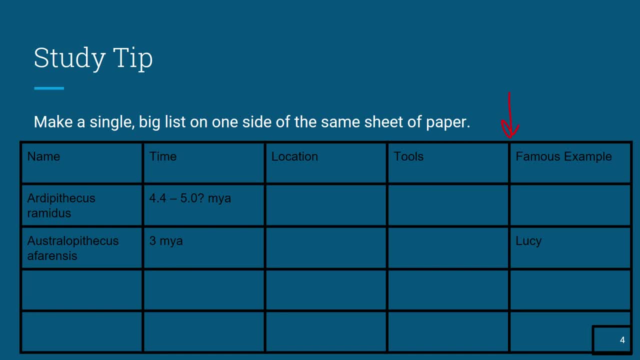 And you will put whatever boxes work best And make the most sense for you right, But at least have those five right, And so you'll have to know. You know Australopithecus three million years ago I think. there wasn't a location on him, He didn't have tools. 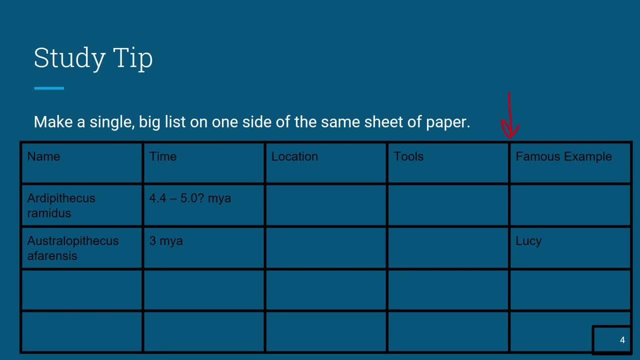 The famous example is Lucy. right? Those are the key things to know about each species, And some of them will have, you know, maybe a sixth category. You can maybe just put miscellaneous, as like a sixth box, Whatever works for you, right? 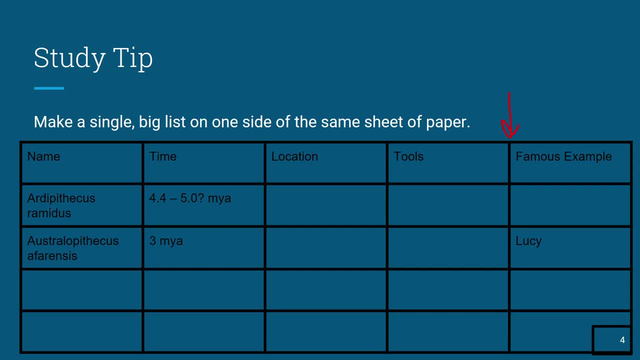 But have it all, Yeah, On one sheet of paper. The reason this works so well is if it's on several pieces of paper, you'll have to kind of flip back and forth And your brain sees them as separate images and separate topics, almost At least for me personally, I found, when it's on the same sheet of paper it's weird. I almost remember like their order based on like which one was above it and which one was below it. 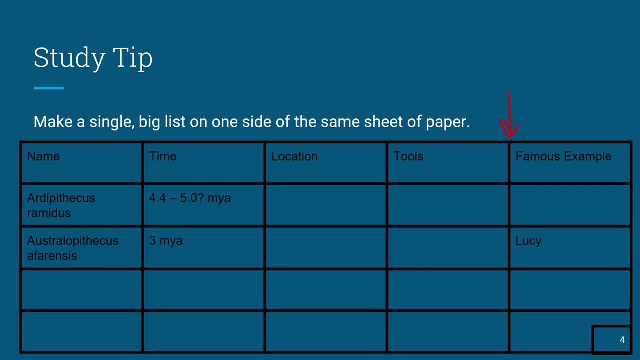 So I made this chart And then when I went and took the test, I could actually picture it in my head on one sheet of paper, because I didn't have to flip back and forth And I almost just cheat sheeted out of my brain. I had memorized this chart. And again, it was because I made it now, not three days before the test. 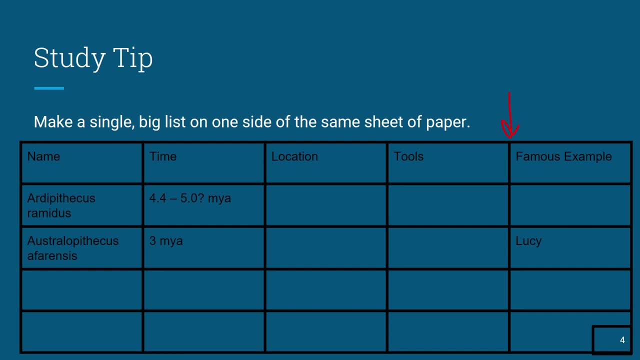 Even though we haven't talked about all the human, pre-human species. it's in his PowerPoints, right? So go the extra mile a little bit on this one. Go into the PowerPoint, Go into the PowerPoints And they're all just right there. It's not going to take you hours, It can take you 10 minutes maybe, And just make your whole chart with all the species from his PowerPoints, all their key information, and then start memorizing it now, Because I promise you there will be questions about that exact information right there And if you've just glanced at it or looked at it for a couple days or you remember a few, but not all of them, almost all of them are going to be there. 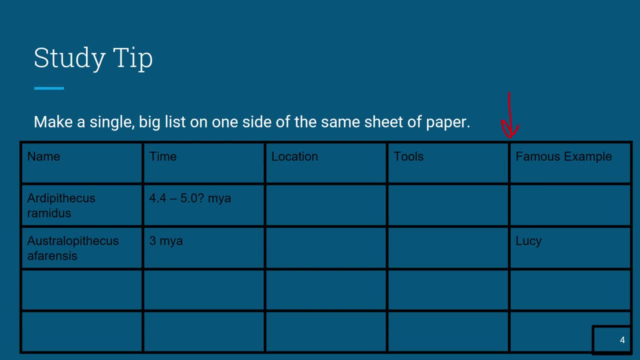 Almost always, the one that gets asked is the one you don't remember, right? You're like, oh, I know everything about Australopithecus. And then he brings up some totally different one. that you're like, oh, I didn't spend a lot of time on that one, right, So know them all, Because none of these are like more important or more test question worthy, right, So know them all And start that now. Okay, Anyway, that's my big log rant, because from here it's basically just memorization stuff. 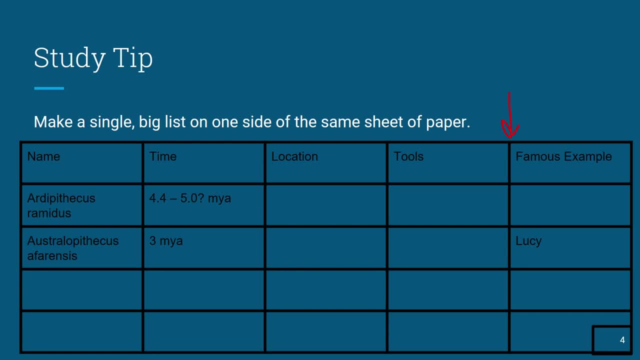 You guys will pretty much come to these sessions from here until exam four for me to reiterate things, because hearing it more than once helps you memorize, And I'll give you some more tidbits and facts like this, right, But there won't be any like really big concepts that you have to like know the math behind or anything like that, right? So start just getting into memorization mode, Okay, That being said, 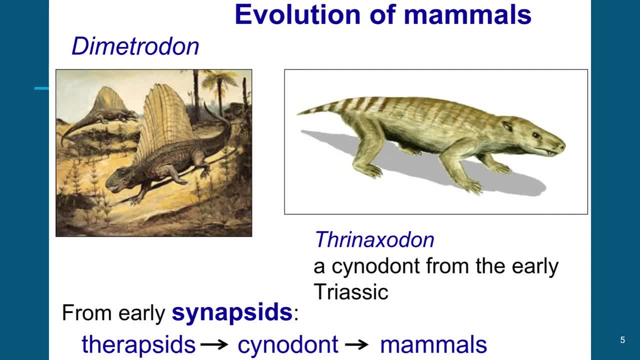 let's get started. So how did we before we even get into pre-humans, how did we even get to mammals at all? There are a few key transitional species that we talked about in class. So how it started was the synapsids right? The therapsids became synodonts. The synodonts became mammals, Yeah. 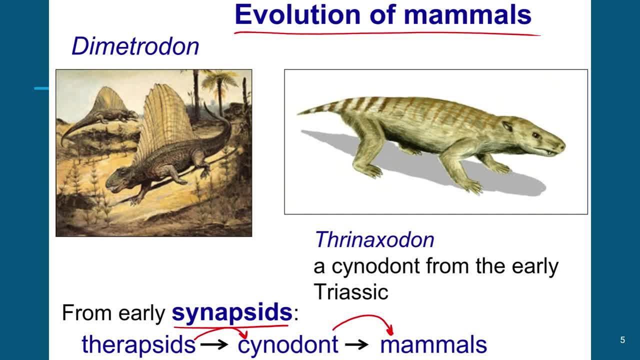 I believe therapsids are a type of synapsid, but I could be wrong on that. I don't think mammals are synapsids. I think it goes synapsids, but inside the synapsids is therapsids to synodonts, to mammals. I'm not 100% certain. So if anybody finds out, 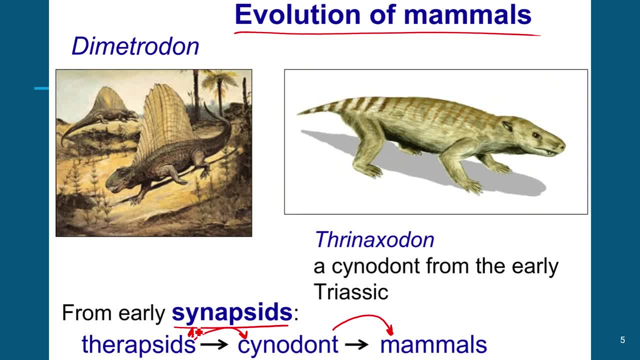 but pretty sure. it's just that therapsids are a type of. So the classic examples that you need to know of are the Dimetrodon and the Thrinaxodon. I always have a hard time with that. one Just know that they're transitional species going from synapsid to mammal right. So I don't know for sure, but I would guess he's probably a therapsid. 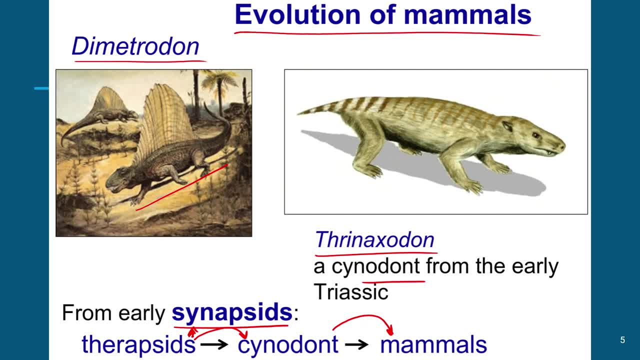 I don't think you have to know that. And then Thrinaxodon followed as a synodont and then eventually we got to mammals. So know these three terms right and the order that it went- Therapsid to synodont to mammal- Make sense? Any questions? 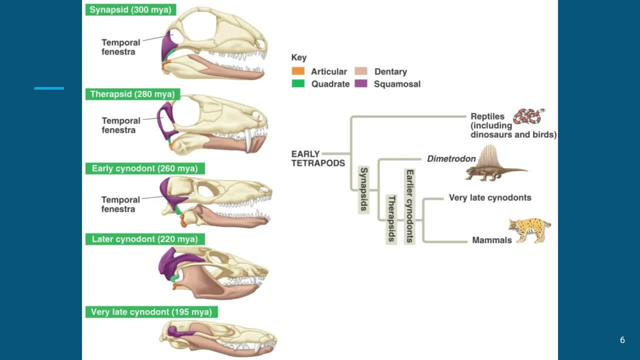 Okay, Tell, this is by skull shape, and that's actually where the- what am I trying to say- It's where the names come from- is based on their skull shape. So the synapsids, right, had this single hole behind the eye. The therapsids, if I remember right, had it on both sides. This isn't like test stuff. 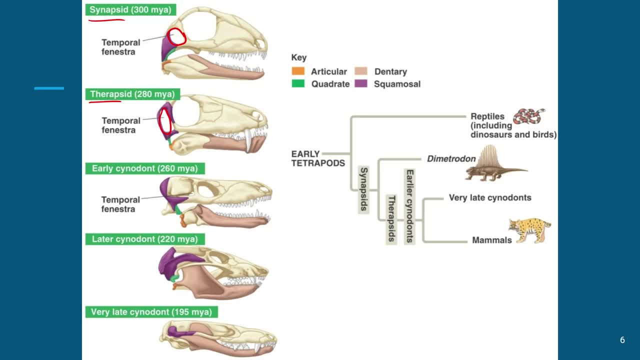 The number of holes isn't test stuff, The naming and things like that is So the synapsids had that one hole. Therapsids, I want to say, had the two. Then the synodonts: they still have the same one, but you can watch it flatten out and get a lot smaller. Then the later synodonts- I believe it would be this area there- And then the very latest synodonts. I can't even see one. I think they may not have one at all, And so they're able to watch skull shape. 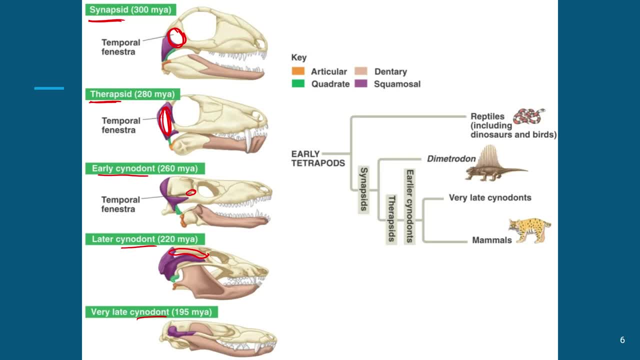 Change from synapsid you can think of maybe just your standard dinosaur- right into what became the mammalian skull shape. Obviously, not every single mammal has that skull shape- Most don't- But it's some variation of that And they're able to trace that lineage. So test questions on something like this would probably be just along the lines of either knowing that 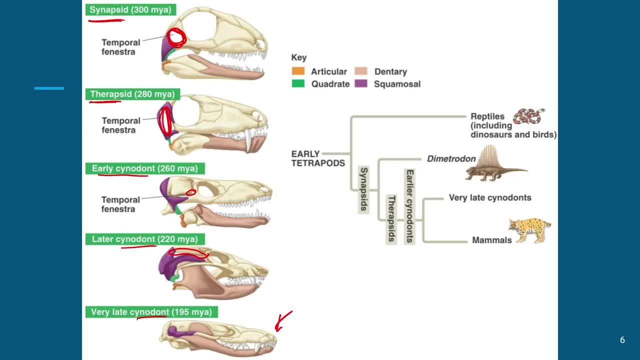 the location and size of the temporal fenestra is how they were able to figure out the lineage from synapsid to mammals And again just that order, Synapsid. So I guess I was wrong. It goes synapsid then therapsid, then synodont then mammal. So therapsids weren't a type of synodont Synapsid, they were the species right after. 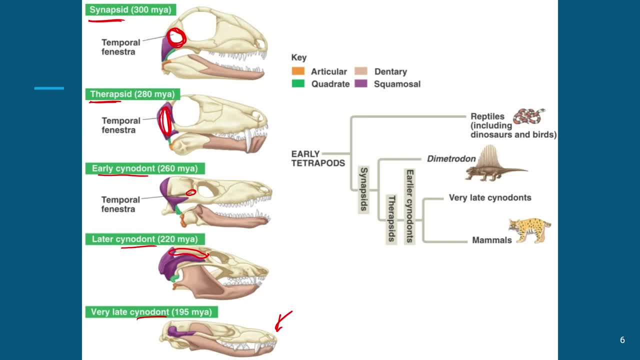 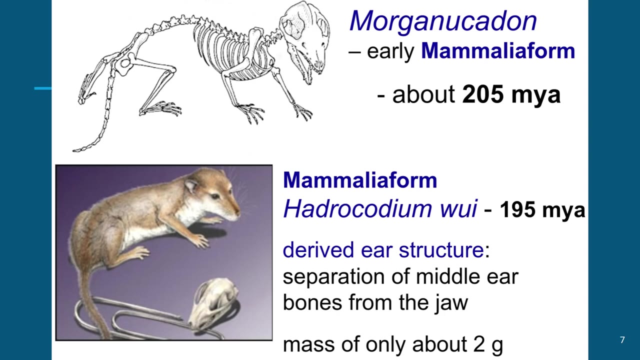 Yeah, that's what I would know about this part. Make sense to you guys Feeling okay with that? Okay Again, this is all just about knowing the examples, right? Dr Messina loves examples, So the famous transitional species you need to know: morganucodon. 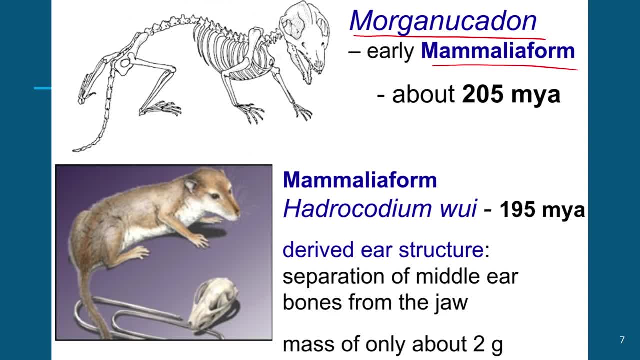 It was the early mammalia form. So from what I understand, it wasn't technically considered a mammal because it's a transitional species, but it's mammalia form in the sense of it was. it looked a lot like a mammal, It just didn't quite have every single characteristic, right. Yeah, so I would just know morganucodon was a transitional species for mammals. 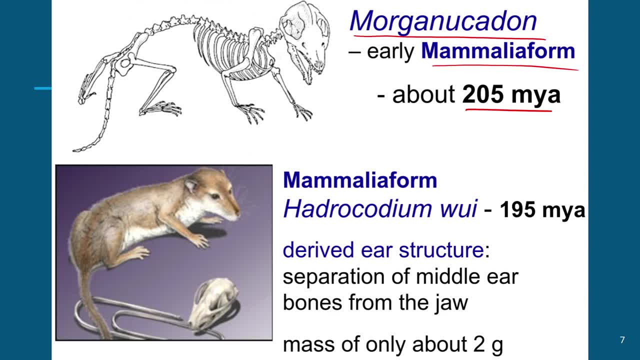 about two years ago. Yeah, 205 million years ago. I don't know that we talked about Hedrocodium Wu all that much. If you happen to know that name and date as well, it wouldn't hurt you. You wouldn't need to know that it weighs two grams or anything. 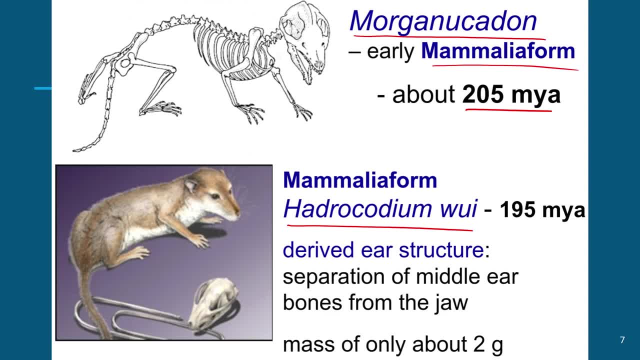 I would be shocked if Dr Messina asked that on a test. So anything's fair game, though technically Don't come to me and be like you. said that he wouldn't ask if it was two grams. I said I would be shocked if he did. 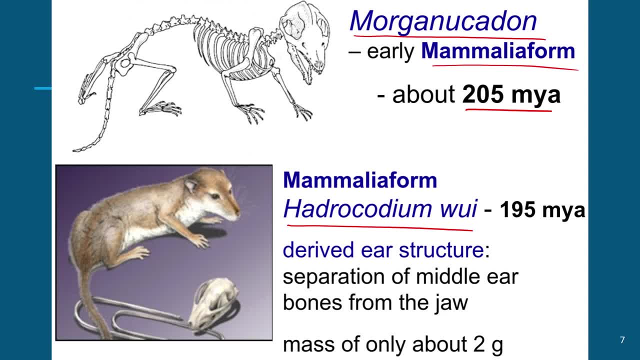 And it's recorded on video as proof. So when I get an email, I'm just going to reply with these 30 seconds from this pen and I'll just send it to you. I told you that it could be on there, All right. 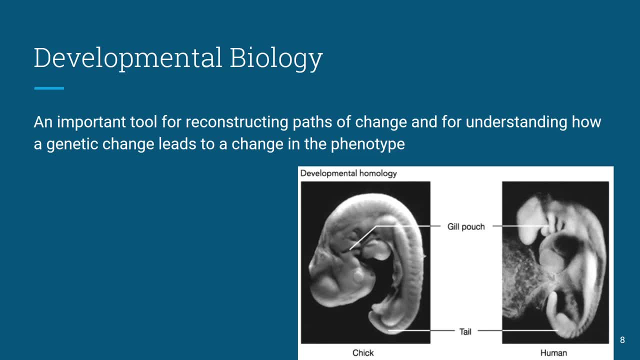 Developmental biology is what it sounds like, right. It's the study of how living organisms develop from zygote, Zygote to essentially all the way up to sexually mature organism. So it helps us understand how genetic change changes phenotype. so how genotype affects phenotype, right? 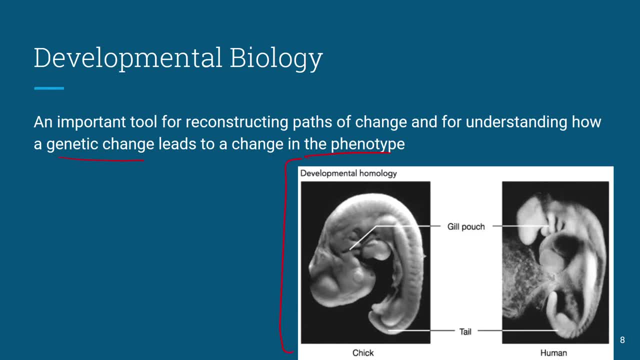 One important thing is: most animals look the same for the first few days, even up to weeks, right? If those weren't labeled chick and human, would you be able to tell me which one was which? Not a chance, right? They don't even really look like anything. 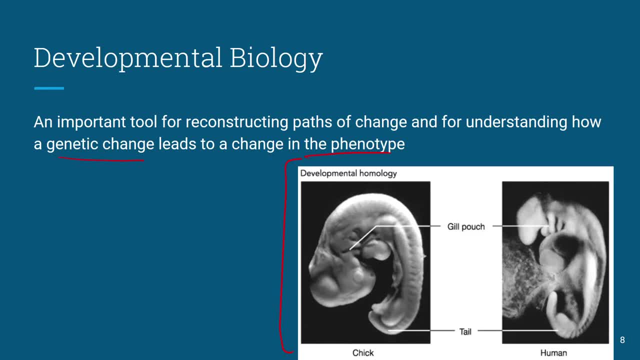 They both have a tail. They have gills- right, But neither chickens nor humans have gills when they're born right, except in extremely rare cases, And just in general they follow all the same body plan, right. This is just because all vertebrates came. 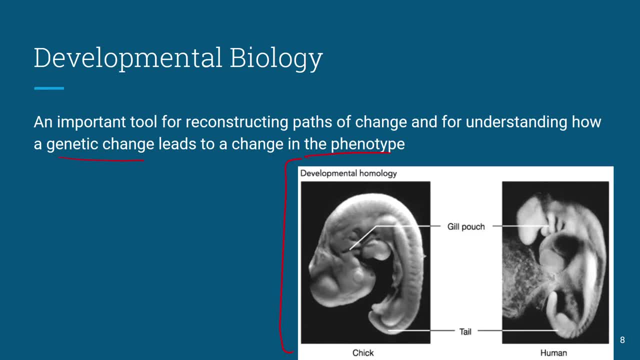 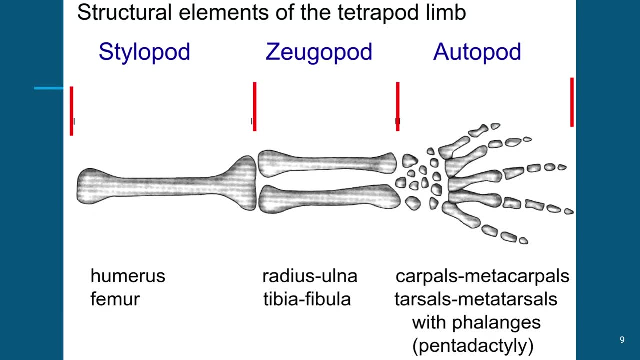 from the same ancestral species, right? So they all share the same Right. They all share the same building block, if you want to think about it like that, right? So something that was important in developmental biology was looking at bone structure, right? 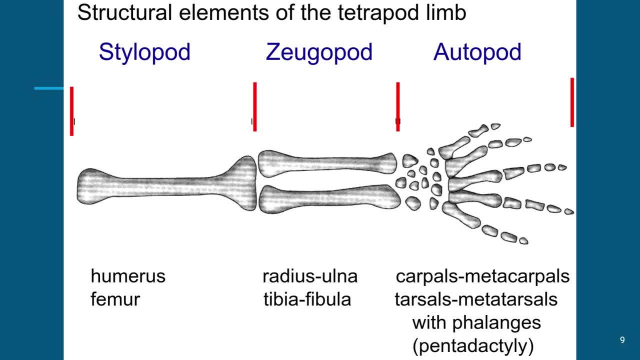 This helps identify different species and what kind of class and genus and family they can fall into can be based on bone structure. So these are definitely, definitely names you need to know. I remember a test question. I don't remember which of the three it asked me about. 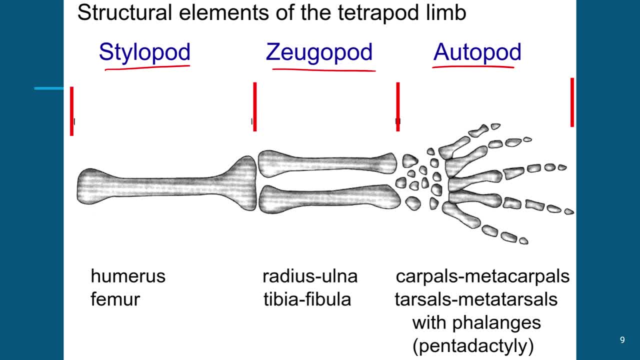 but I remember a test question essentially asking where one of those was located. I don't remember. So if it was like the autopod in humans is the hand, or the zygopod is the forearm or the stylopod is the bicep area, 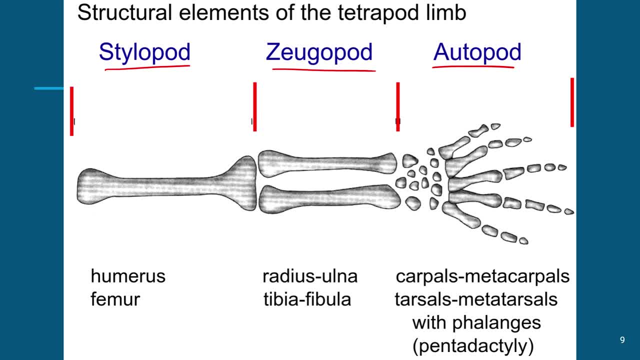 Does this have a regular arm? Pre-arm Arm Arm- It's arm and forearm Two arm Humorous, Yeah, And notice it says humorous and femur because this isn't exclusive to arms, right? In fact, most animals don't have arms per se usually. 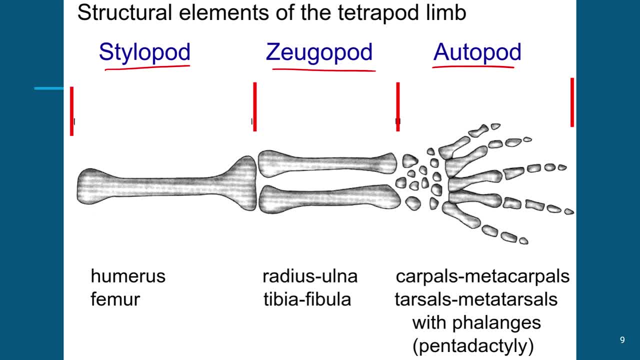 just multiple legs right, So it also works for femurs, tibia, fibia, tarsals, metatarsals right, And it's not just for humans, right. Dogs have a stylopod, a zygopod and an autopod. 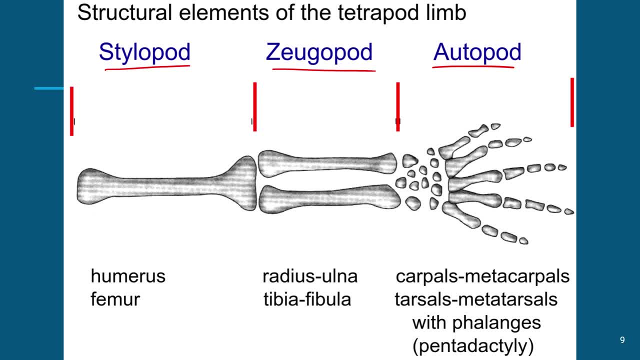 Right, Any tetrapod, so any four-legged creature, has this bone structure, right? So just know, stylopod, zygopod, autopod, right. I don't really have any good tricks for remembering this. I do always remember that autopod is the hand. 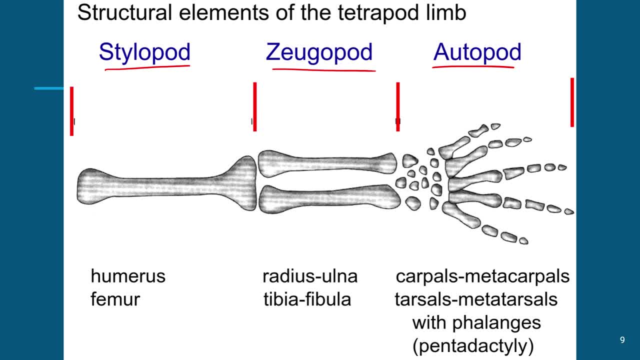 because if you drive a car, you're auto, which ironically it would be manual, Right, But you use your hand right. So that's just how you drive your auto. if you're British, I guess with your hand right. 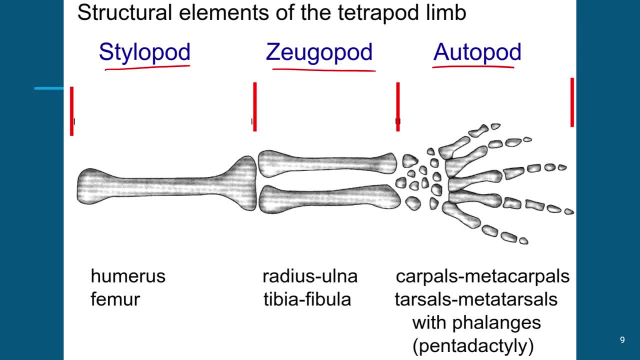 Stylopod, zygopod, I don't know. Yeah, I have an idea. Yeah, I feel like with the stylopod you get like a stylus and the stylus is just a single bone. Oh yeah. 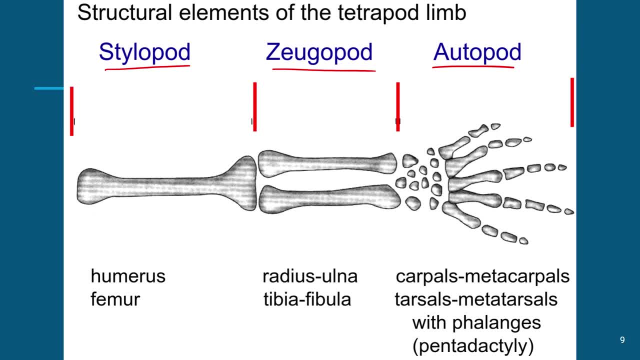 A single bone Right. yeah, the one bone right is your stylus. If you go with zygopod, the z kind of looks like a two. Oh yeah, Yeah, you could say the zygopod is like a z right there. 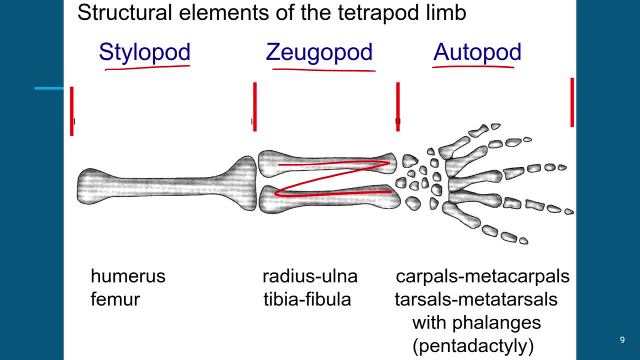 Look at that. you guys did great And autopod is the car which makes no sense. But in my head I was like: that makes sense. You drive your car with your hand, So if that doesn't make any sense, 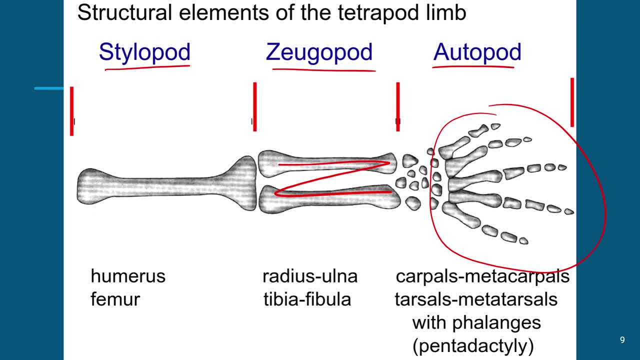 you make up your own thing. right, A pod which could contain a lot of stuff in it. A pod has a lot of stuff, a lot of little bones, right? Or you could you hold your iPod in your hand, even though, oh, they all have a pod. 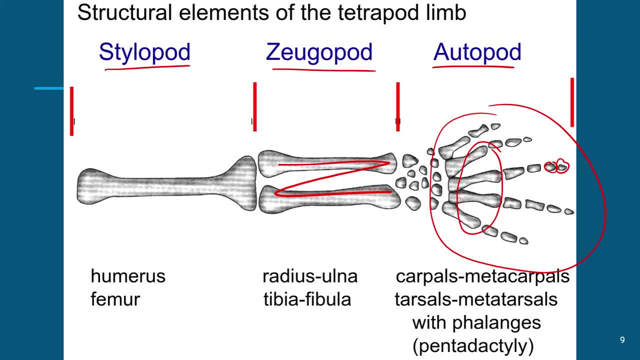 I ruined it. Plus, nobody uses iPods anymore. Do they even sell iPods anymore? You still have an iPod. I still have a. What the heck man? Yeah, so come up with your own way of remembering that. Just make sure you know: stylopod, zygopod, autopod. 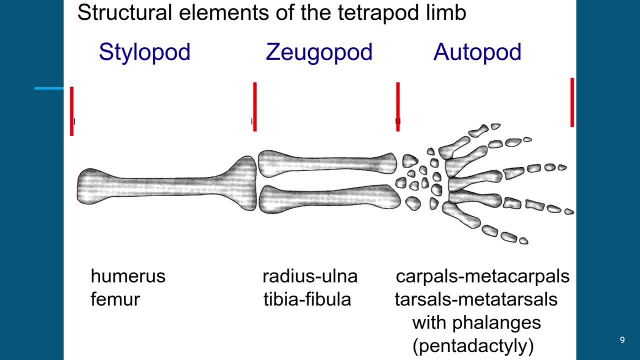 where they are and more or less like the structure. So if it said the autopod is also known as the hand, or the stylopod is also known as the arm or the zygopod, The zygopod is the forearm, or which bone maybe you? 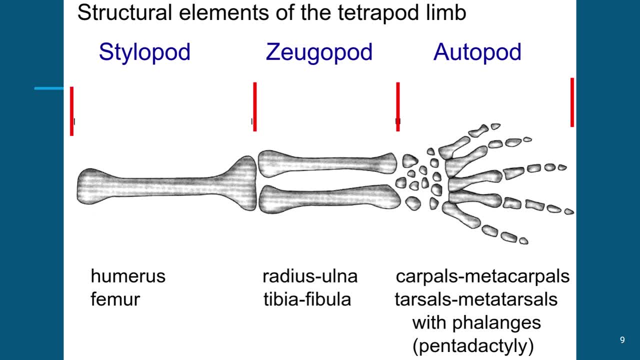 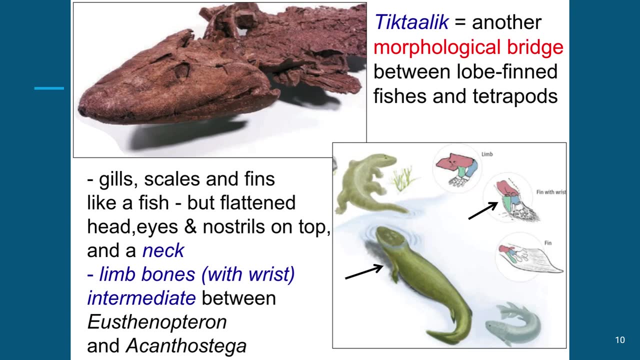 could relate it to. So your stylopod would be your humerus, something like that. right Make sense, Yeah, OK, So now we get to start looking at how we got to the tetrapod limb as it is now. 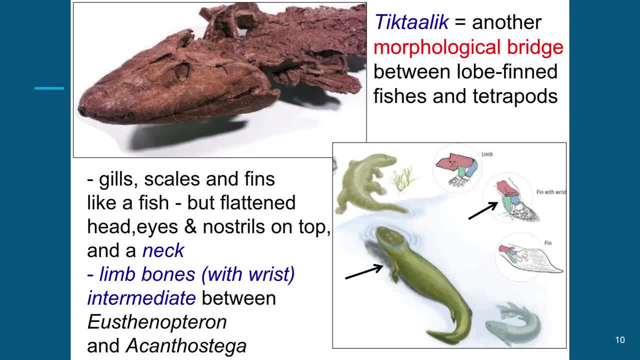 especially pentadactyly. so five fingers Again. important transitional species. Whenever you see the name of a transitional species, you have to know it right. So Tiktaalik was the bridge between lobed finned fishes and tetrapods, right. 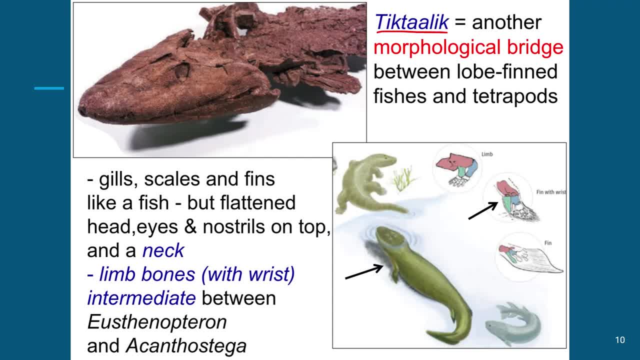 It's what took certain fishes from having just a fin with kind of one bone in it. I think that's how they were into eventually what became arms and legs, right? Other important things? OK, OK, All right, All right. 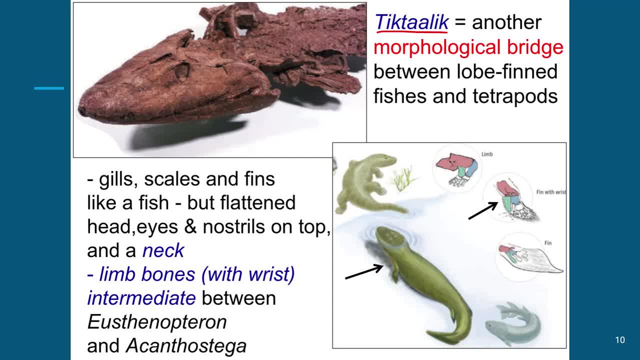 All right Features to notice were flattened head and eyes and nostrils and a neck right. Fish don't have flat heads with eyes and nostrils on top and a neck right. That's what amphibians have, So this Tiktaalik was going from fish to amphibian. 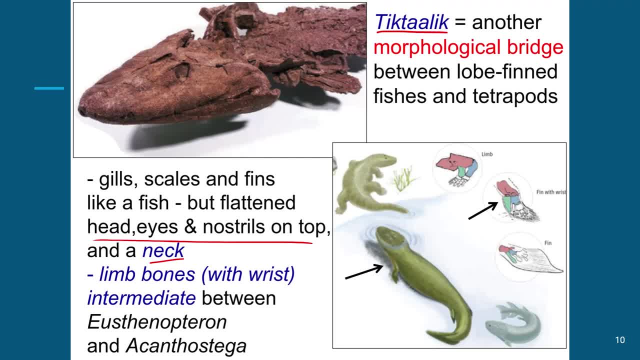 And he was changing his physical shape. right, His limbs had a wrist. Fish don't have wrists, right, They just have a fin. Yeah, What are tetrapods? Tetrapods? Yeah, Tetrapods. Four limbs. 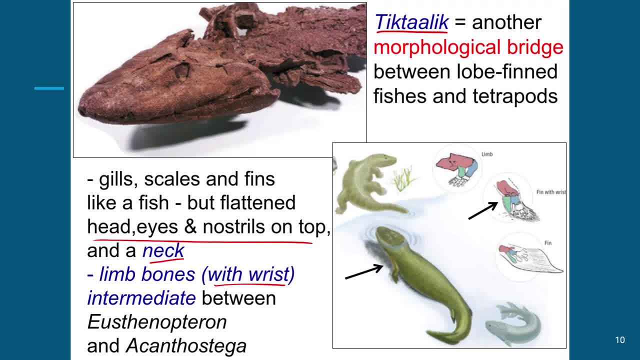 And I don't know if exclusively they have to have five fingers, but they most of the time do So. tetrapod just means four legs. I don't think they have to have five fingers because of horses Right Horses just have one. 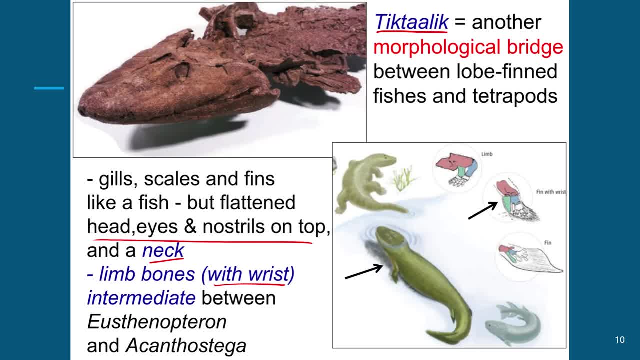 So, yeah, Most of the time they're pentadactyls, but they don't have to be. It's just if it has four limbs with a stylopod-zugopod-autopod is what makes it a tetrapod. 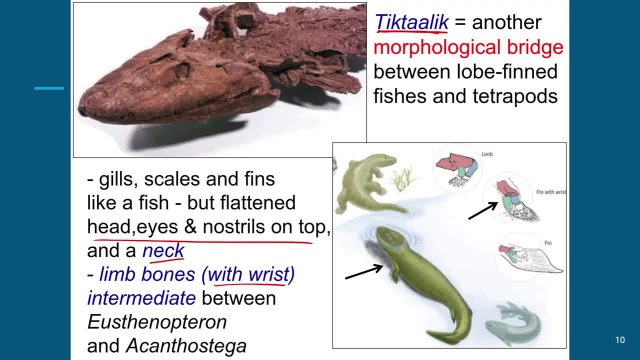 So Tiktaalik was not a tetrapod right. He was just on his way to a tetrapod right, So he had a wrist, but he may not have had the full stylopod-zugopod-autopod. 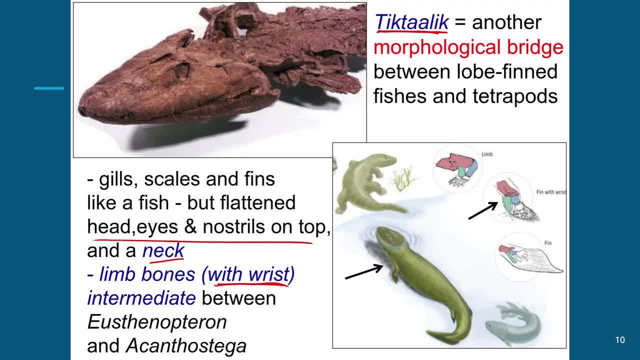 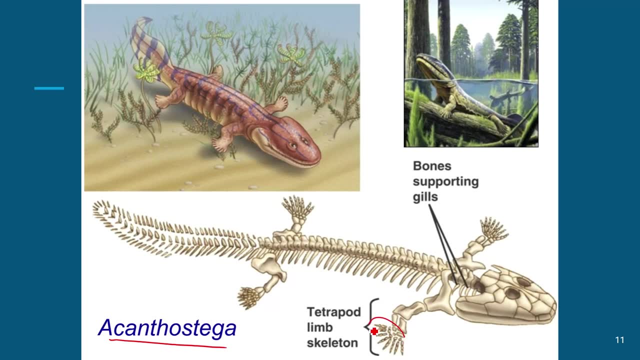 something like that. I'm not even sure, But just know Tiktaalik Intermediate between fish and essentially amphibians Sound good. Acanthostega is an interesting one because he had, I want to say, eight fingers, Yeah, eight. 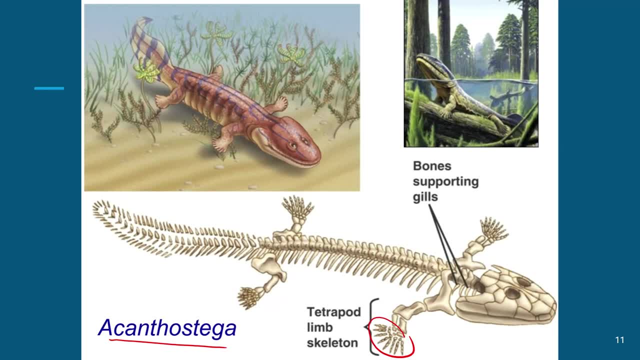 And Dr Messina mentioned that when they found this fossil, they thought that two fossils had formed on top of each other, because they were like: why does it have so many freaking fingers? But the more they dug them up and found them, they realized no, these all just have eight fingers. 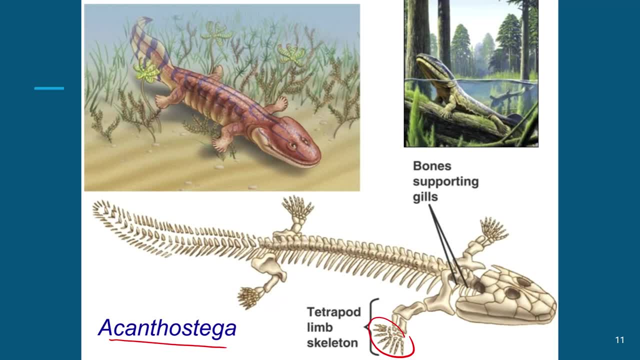 They don't really know if there was a specific reason why, but that's just how they looked right, So you can even see it looks weird. It looks like a little alien hand. He's got just tons of fingers right. They were. I don't know if they were a transition. 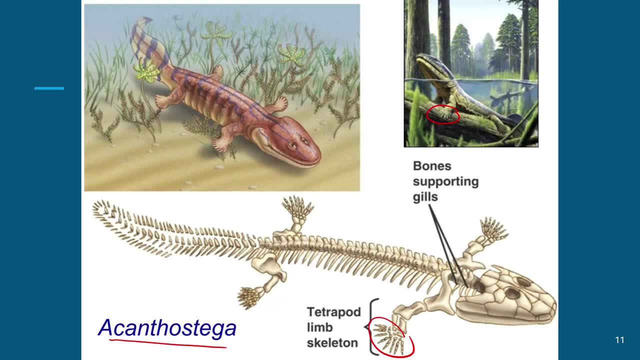 between fish to amphibian, or if they were fully formed amphibian. But again, they're going from fish to amphibian, Right, Yeah? Yeah, They may even be all the way there. So Acanthostega was just an interesting example. 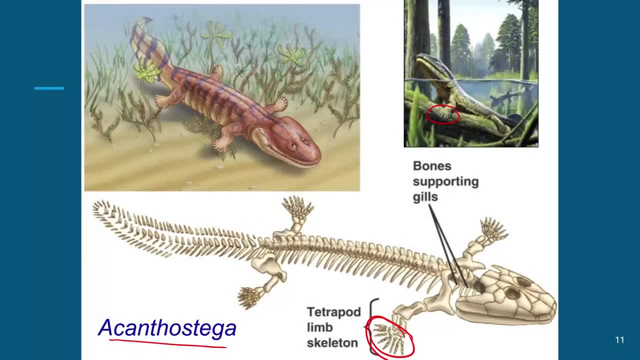 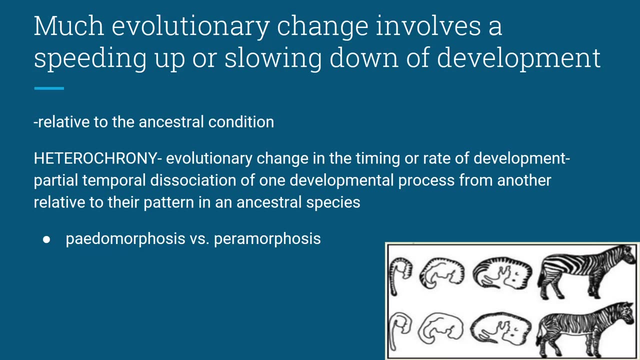 because of not Pentadactylus tetrapodalum, Sound good, All right. So a lot of development. well, I guess a lot of evolutionary change is just messing with, tweaking with development in utero. right, It's just speeding things up or slowing things down. 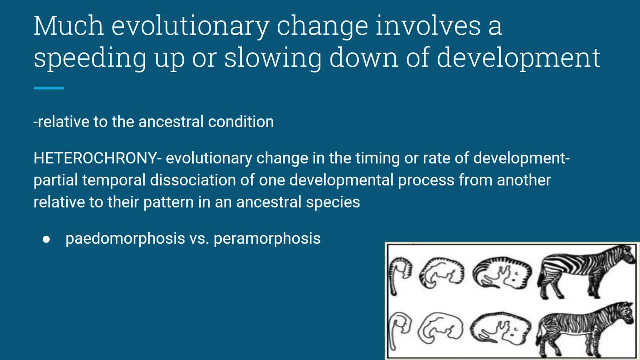 or changing a little bit of this or adding a little bit more of that, right? So a couple of important things to know. First off, heterochrony- important vocab term. It's just change in timing, right? Hetero means different and then chrony means timing. 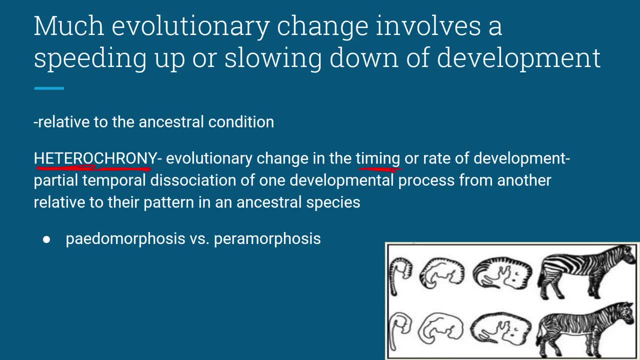 Time It's a change in the rate of development, right, And this can change characteristics on a full organism scale, right? So the example I found online was with a zebra, And I don't even know if this is a real example. 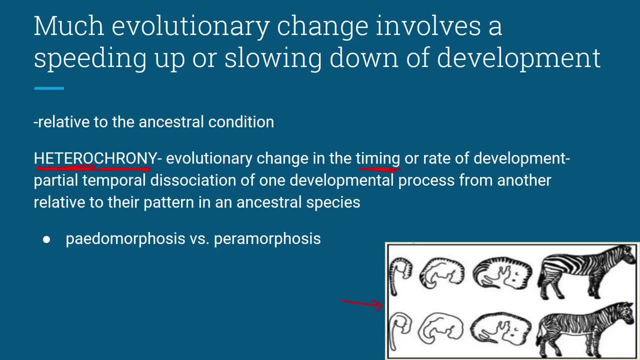 but it gives you a visual right. You take a zebra fetus and if you get it to develop stripes right away, they're a lot thicker. Right, They develop for longer and he gets thicker stripes Again. I don't know if this is actually something that happens. 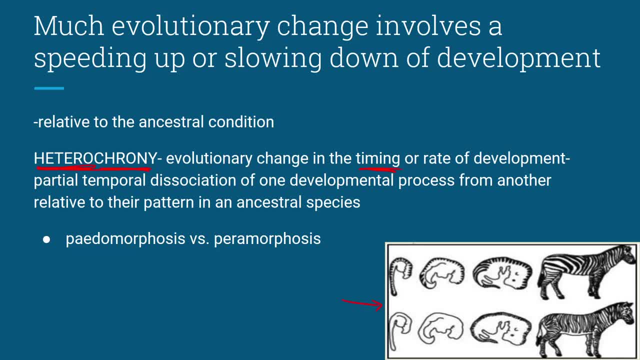 Or you take a zebra fetus and you don't get him to develop stripes until pretty far along into the fetal stage and the stripes are a lot thinner right, And it's literally just that change in when things started developing. Everything else could be exactly the same. 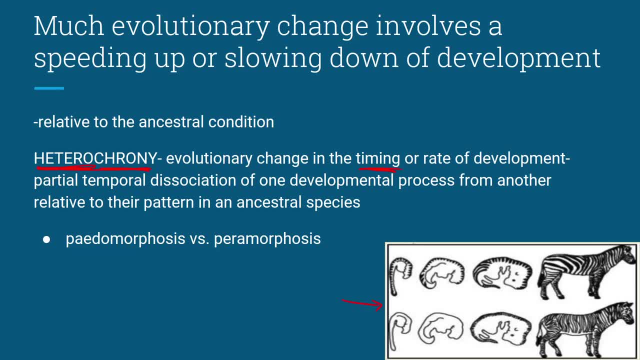 They could be exposed to the exact same hormones. They could even come from the same mother, right. They could even be siblings, right? But if one starts developing stripes later than the other, they'll look different, right? And this goes for everything. 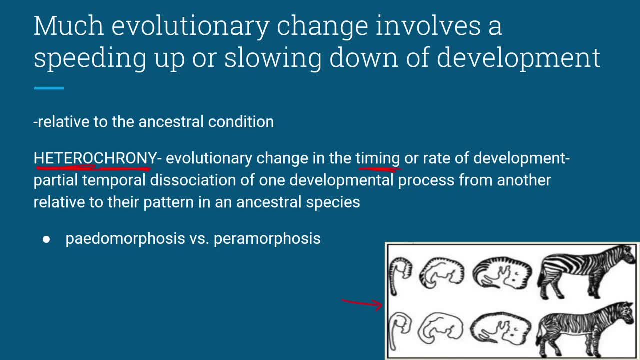 If you change development time, then you change a trait, And it can be huge. It can be brain size in humans, right? That, basically, is what set us apart from every other animal on the planet. Or it could be something as small as stripe thickness. 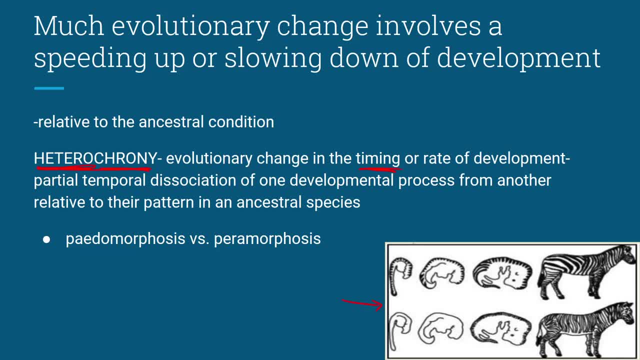 But it's just that change in timing, heterochrony. It's just that change in timing, heterochrony. You guys good with that. So then we have two more vocab words: pedamorphosis, paramorphosis. 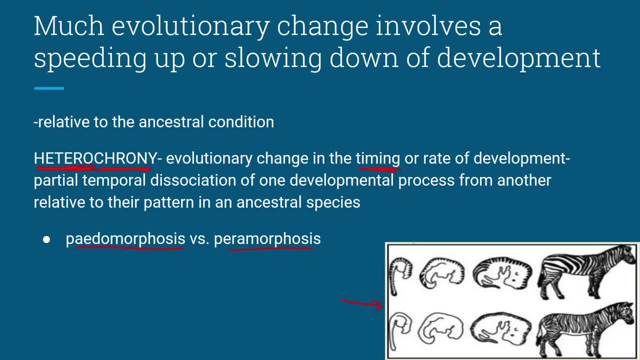 Anybody remember what pedamorphosis is? Yes, Pedo means child, so pediatrician, child, doctor. Pedamorphosis is maintaining those juvenile, infantile, baby Traits right. Paramorphosis, then, is just the exact opposite. 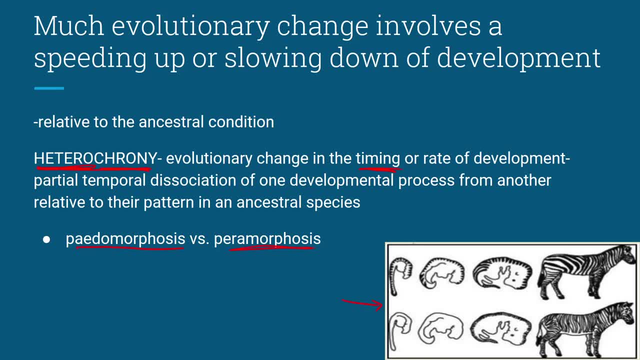 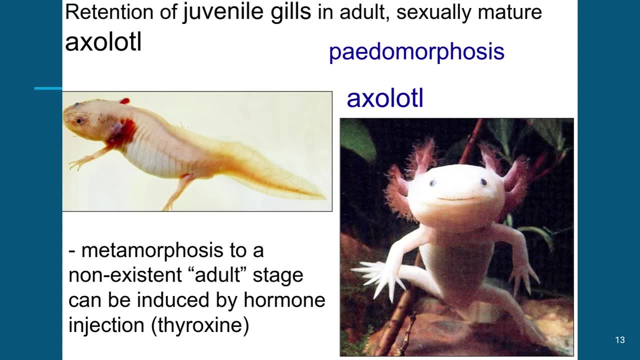 is putting on adult traits more quickly. So some examples of pedamorphosis. is this Mexican axolotl? cute little guy. He still has his external gills, right? This is not normal in salamanders, right? They usually internalize that. 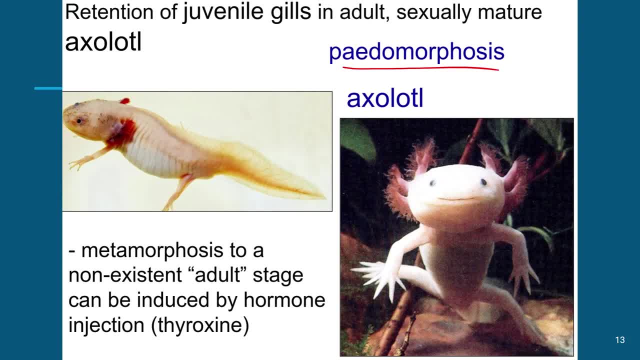 So that when they climb out of the water they don't suffocate right. They have their internal gills, They can breathe water and air right. Axolotl, on the other hand, stays in his juvenile state, But it's a permanent juvenile state. 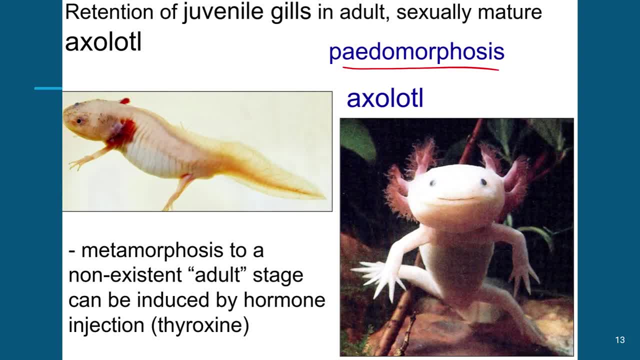 So you can't really call it a juvenile state because he never leaves it. But relative to other species in his family, he stays juvenile Right. They know that this is a juvenile stage because they inject them with thyroxine. It's just a hormone. And they will actually develop into an adult stage that doesn't exist in normal natural axolotls. They can actually kind of force it to turn into an adult that it never would turn into So kind of wild right. They just take these guys, inject them. 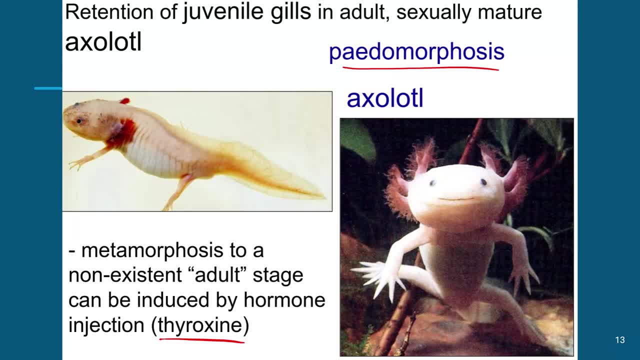 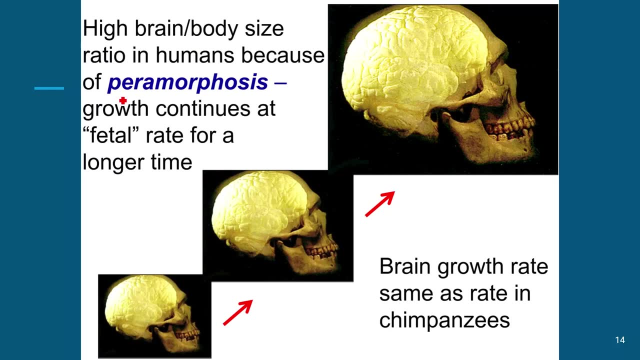 and they evolve like Pokemon, right, Pretty sweet. So yeah, that's an important example of pedomorphosis that I would know: the axolotls and their permanent juvenile state. Then you have paramorphosis in humans, right? 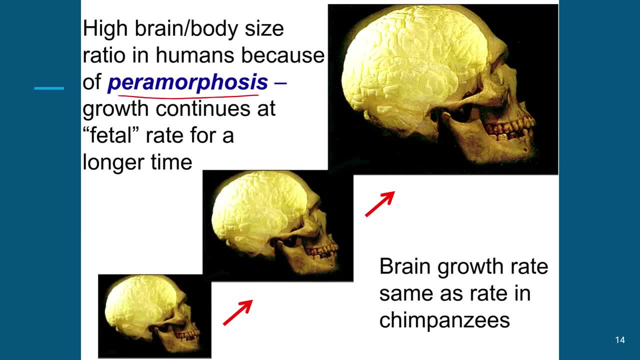 Is the fact that you maintain your fetal growth rate into adulthood, And that's why humans and a lot of primates have a really high brain-to-body size. Our brains are much larger compared to our bodies than most animals, right, Especially like millions of years ago. 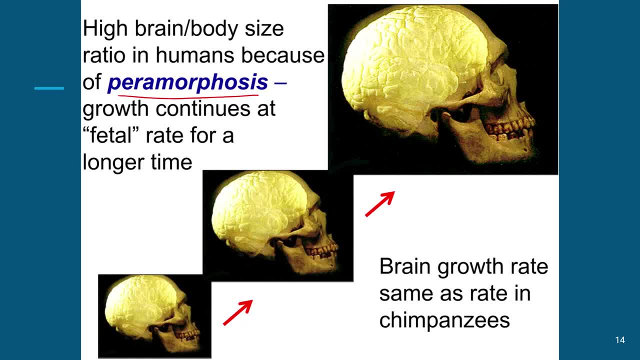 Stegosaurus had like a peanut-sized brain, but they weighed hundreds of thousands of pounds. right, We're the opposite. Our brains shouldn't be as big as they are, But because of paramorphosis, we keep developing our brains as fast as we did, pretty close to as fast as we. 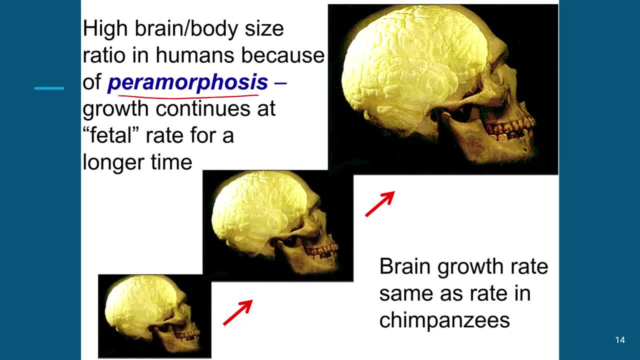 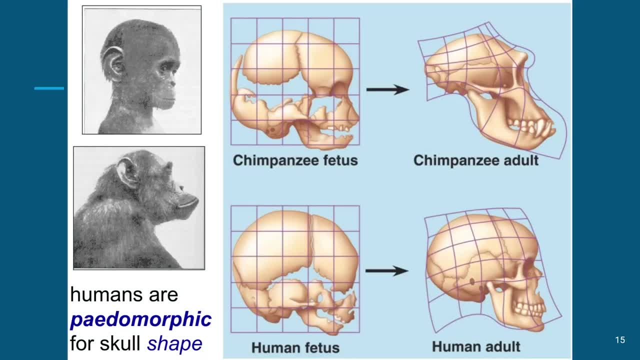 did when we were a fetus. Make sense, Everybody follow that one. But you also see pedomorphosis in apes, Sorry, in humans. So the pedomorphosis, the paramorphosis, is that the brain keeps growing at a fetal rate. 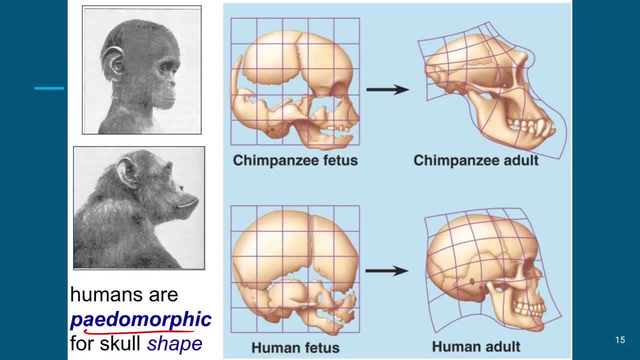 but we're also pedomorphic because our skull doesn't change that much from the fetus. So you take a chimpanzee fetus and a human fetus pretty darn close in skull shape, right General skull structure. But a human adult doesn't change that much relative. 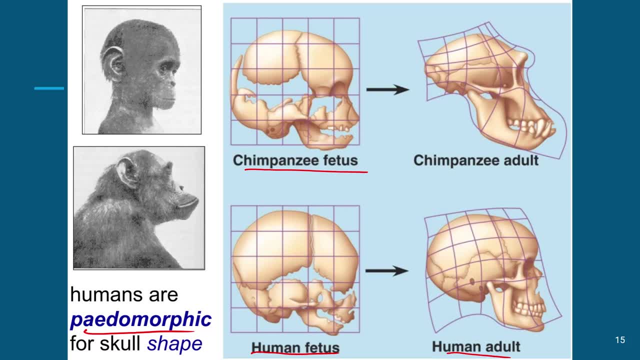 to its baby skull, right, You know, the jaw juts down a little bit, the skull pushes back a little, the front pushes up a little, but not much. You can see it with this. I don't know what that's called. 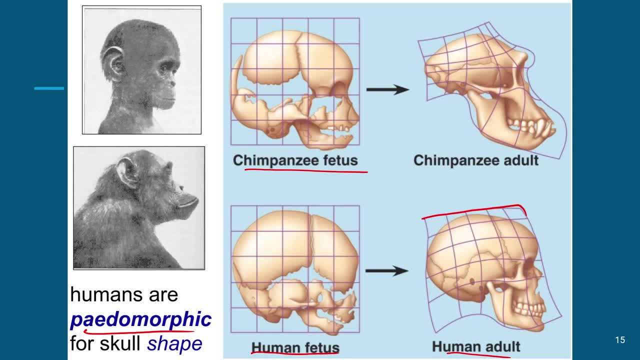 plane that shows you. it only warps a little bit, But a chimpanzee fetus and a chimpanzee adult don't even look the same right. The skull elongates, the brow pushes all the way up and it pinches towards the back and it completely. 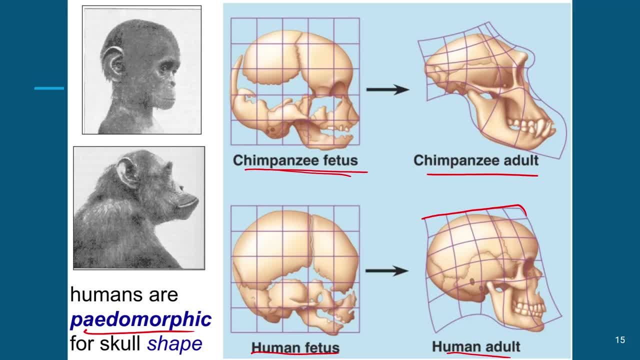 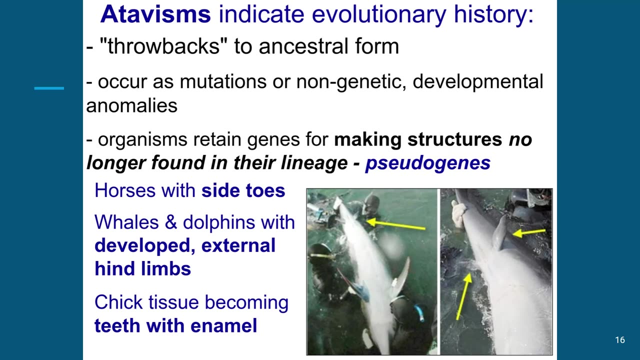 changes skull shape. So that's why humans are considered pedomorphic for skull shape. Cool beans. One person acknowledged me. Good enough, This is the event thing, vocab thing, Vocab term that I find really cool: Atavisms. 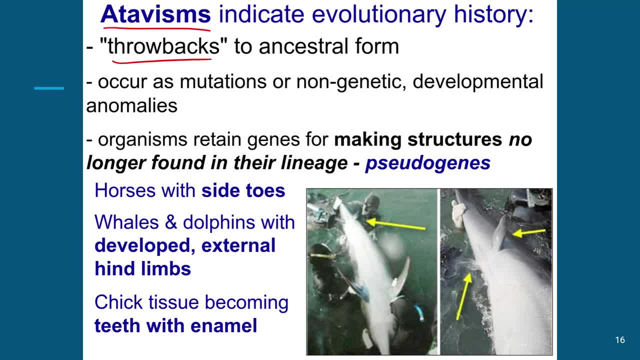 They call them throwbacks to the ancestral form. right, It's when you can watch an organism and all those organisms- dolphins- all look the same, right. But then one random dolphin, for whatever reason, activated an ancient gene from when it had hind limbs, right. 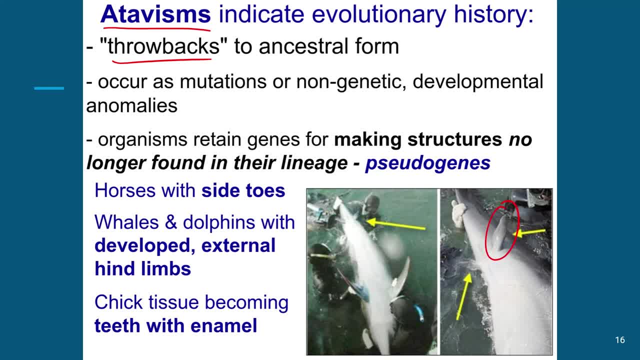 Because dolphins used to be land creatures- obviously not dolphins, but pre-dolphins used to be land creatures, kind of almost wolf-like right. They had hind limbs And for whatever reason, this dolphin happened to activate the gene that told it to grow hind limbs. 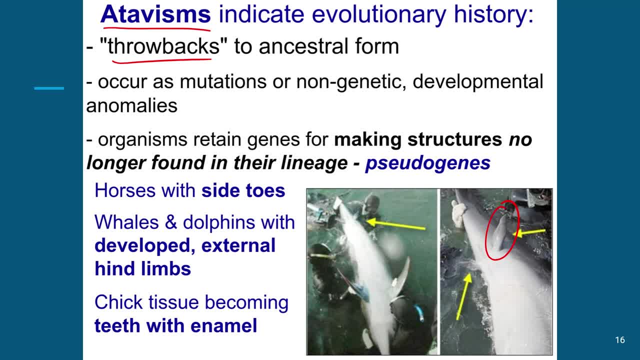 And all of a sudden it had those rear fins And these fishermen were like what the heck? Dolphins don't have rear fins. Is it like a fish that bit it and stuck to it And they couldn't figure it out And eventually they just realized this dolphin. 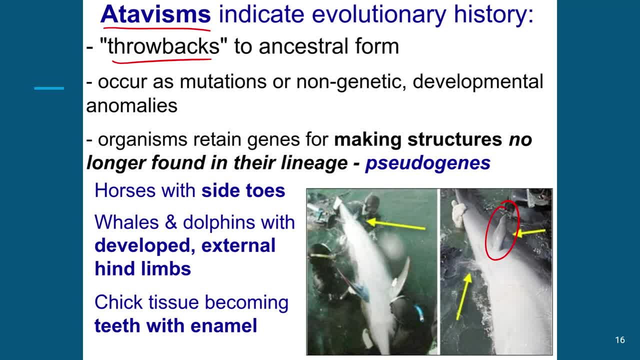 activated an ancestral gene So that dolphin had children. but those children have a greater chance. Yeah, They have a greater chance of having those right? I have no idea. I would guess no, because this is just a totally random event, that out of nowhere it just turns on an ancient gene. 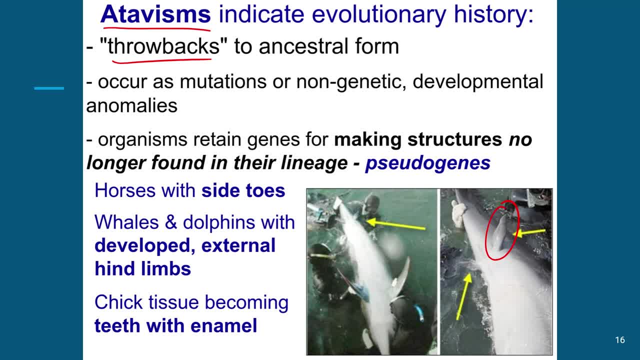 But I don't know if this would affect later generations. That's a good question. Dr Messina would know. So these are pseudo genes, right, They're still there in the genome. They have to be, otherwise it could come out. 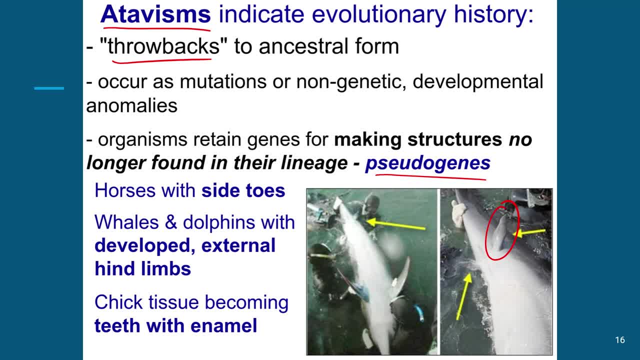 But they don't do anything normally, right? So humans, we still have a gene to grow a tail, right? He showed us a picture of a doctor holding a baby and it has a tail. It was probably like six inches long, right. 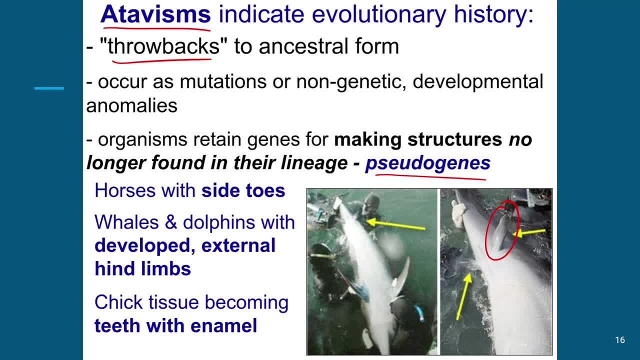 We have that gene. We just never turn it on. We don't need it anymore. but we didn't get rid of it But that baby, for whatever reason, and I don't know, and you don't need to know the underlying reasons behind it. 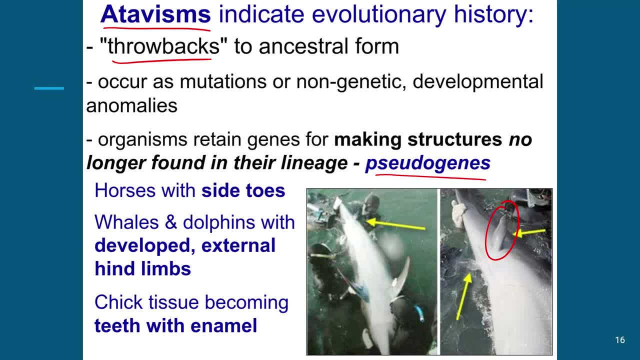 activated that gene and grew a little tail. Those are atavisms. So test question I would expect to see on something like this would be to be given maybe something like which of the following is an example of an atavism, And you're given four or five options. 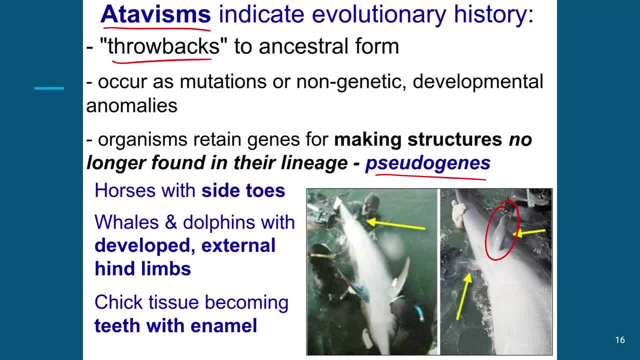 And they all sound like atavisms, but they're not. Or be given four or five examples and they're all atavisms except one right. So let's say like: which of the following is not an atavism? 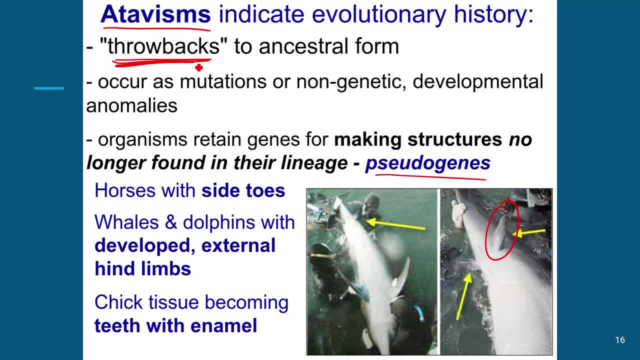 And you would have to know. OK, It has to be a throwback to an ancestral gene from a pseudogene right. So it can't be like a pear tree is crossed with an apple tree and creates the ancestral form of an apple right. 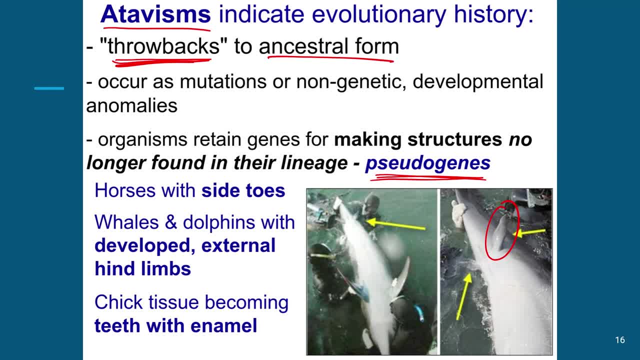 Yeah, you may, that wouldn't work, but in a test question you may have created, created an ancestral apple, But you didn't do it with an atavism, right, You did a crossbreed, So it's not an atavism. 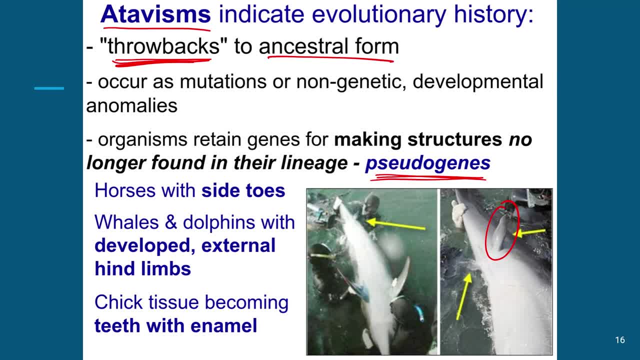 A mutation and an atavism are not the same thing either, right? What's the difference? Mutations, random- These are random as well. Atavism, ancestral mutation: random Mutations are looking forward, right? A mutation happens to an organism. 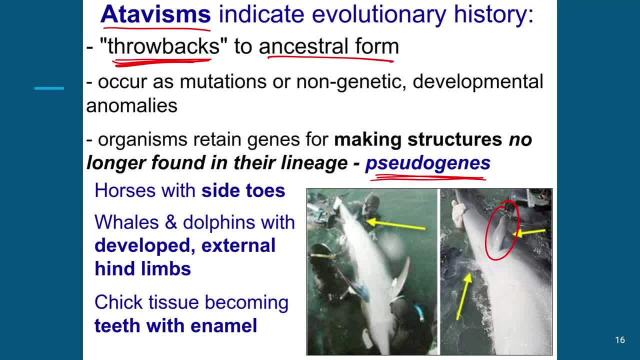 and then, consequently, can continue to affect its offspring. I don't know if atavisms can keep going forward, But an atavism looks backward and it has to work with something that was already there and is just asleep, right. So a dolphin's not going to grow fingers like human fingers. 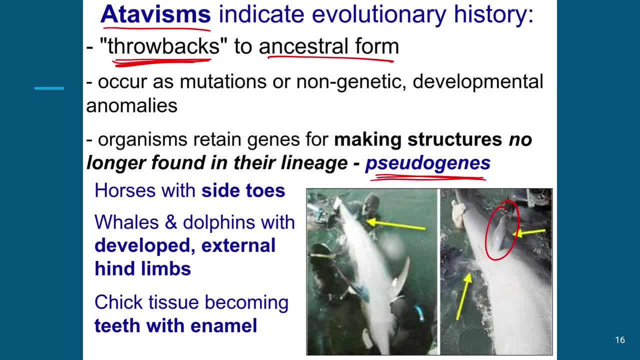 They're never going to grow thumbs and call that an atavism right, Because they never had a thumb gene. So if a dolphin were to mutate and grow thumbs- not an atavism, a mutation Right- Would so like if humans had gills. 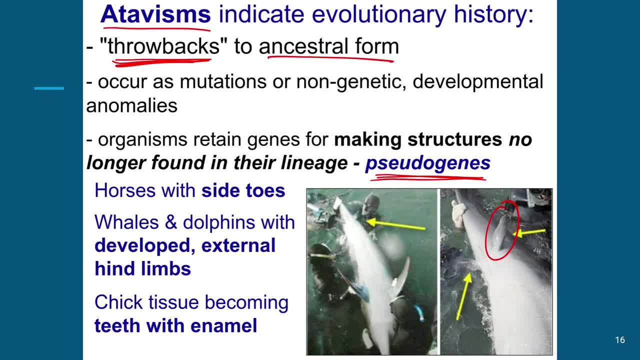 would that be an atavism still, or a mutation? I don't know. It's technically ancestral. Yeah, I don't know. Would it be a mutation if the atavism went from generation to generation to generation, be considered not just a random event? 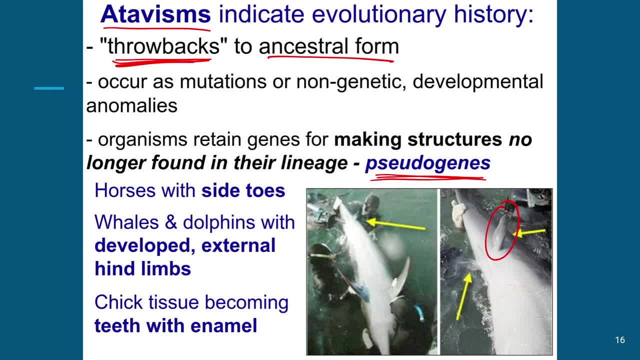 but an atavism that happened. Well, an atavism can't be a mutation, because it's not a change in the genome. It's an activation of dormant genes. So nothing's changing. You just activated a gene that you don't normally activate. 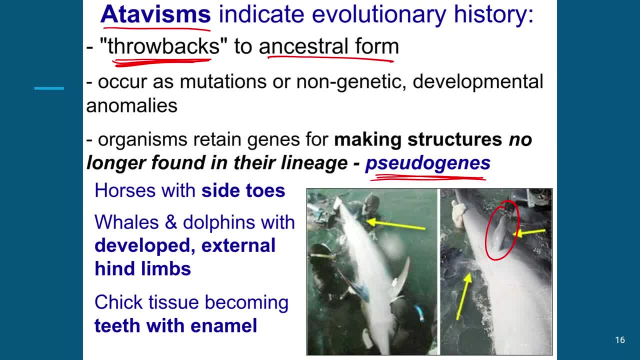 That's the difference. So I don't know with that specific example, because I don't actually know- if humans still have a gill gene. If it were specified in the question, humans used to have, humans used to have a gill gene and now you see a human grow gills. 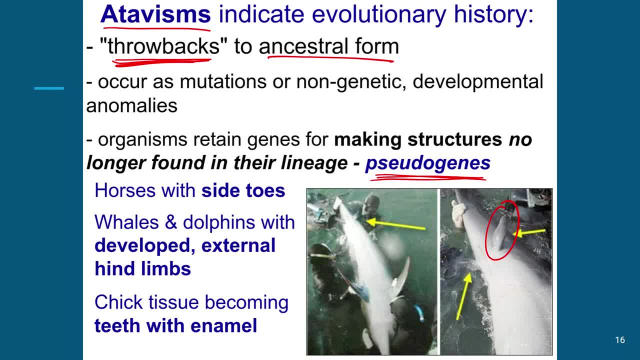 then it's an atavism. Yeah, so if you were to get a question, it would be pretty clear whether or not it's ancestral or a mutation, And that's basically where I would draw the line right: Decide whether it came something already existed. 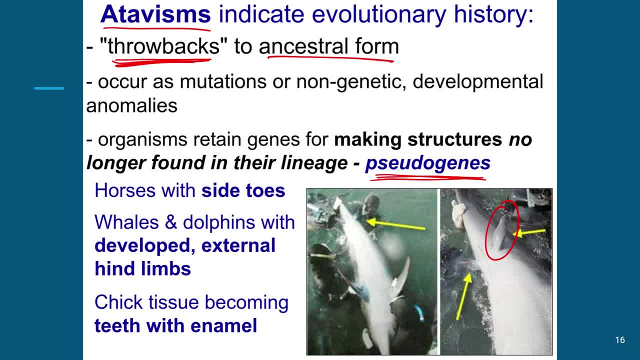 went dormant and then got reactivated- atavism. Or did we take a gene that was already normal and current, put it in the genome and change it and make something new right? So, had dolphins never had a hind limb gene, this would be a mutation. 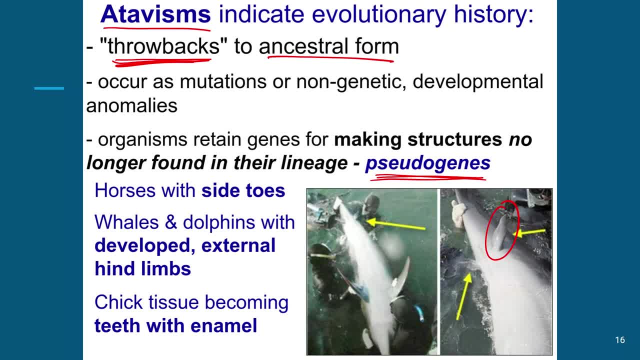 But nothing changed in his genome. you just turned on a sleeping gene, right? Does that make sense? So I imagine there will be a practice test question on this. I would hope Is he going to give us a practice test before, or? 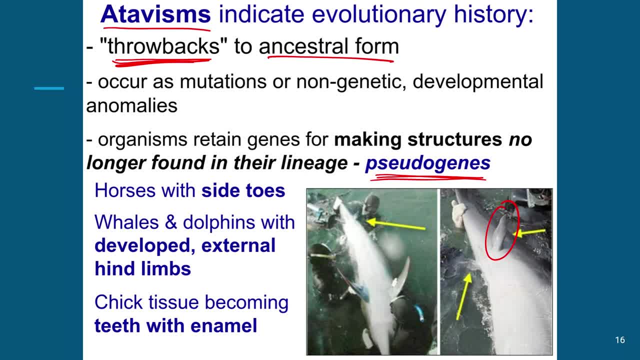 is he going to do the same thing as Bobeck? did only give us the one. What do you mean? Did Bobeck only do one? Yes, No. From what I remember, he did one for exam three and exam four. 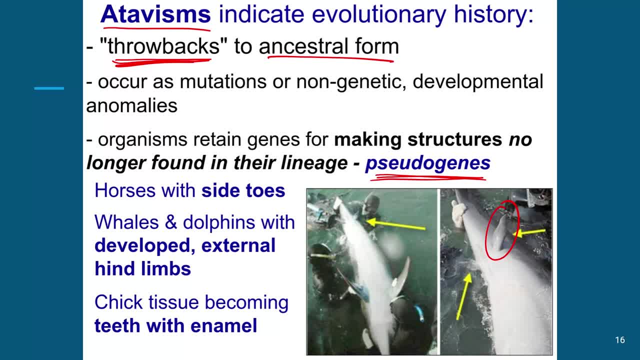 But that's two years ago when I took it. he could change it. That's kind of up to him. Which reminds me. a couple people on my midterm eval asked me if I would make practice tests for you guys. I don't know if you guys remember last semester I tried to and got shot down. 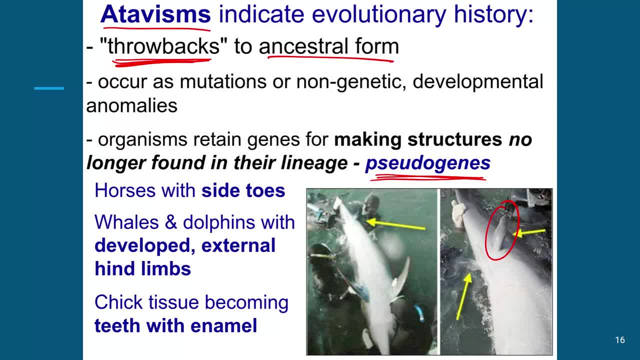 So I I'm not allowed to make practice tests. I'm allowed to make practice questions here in session, but I can't like put together a practice test and and put one out there. I think it's just because the professors would rather do it themselves. 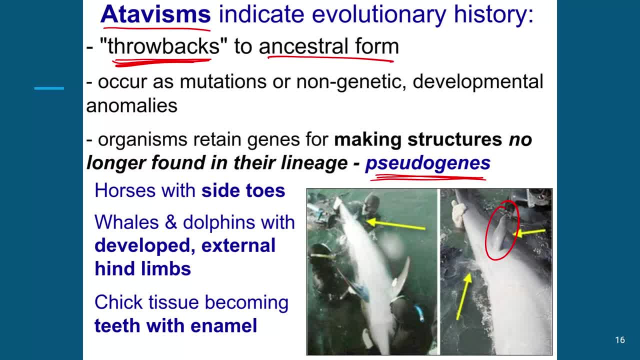 cuz they're the ones writing the test And so obviously their practice tests are a lot more indicative of test material. So it makes sense. so stop asking. No, I only had a couple people who were like it'd be nice if you made practice tests. 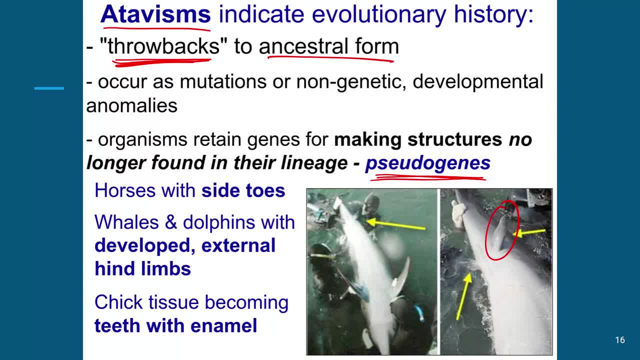 And I was like it would, it would be nice. It would be really nice, Not for me, but for you. I don't wanna do it, But I can. So it's not even that I'm just like I can't. I don't wanna, I can't. 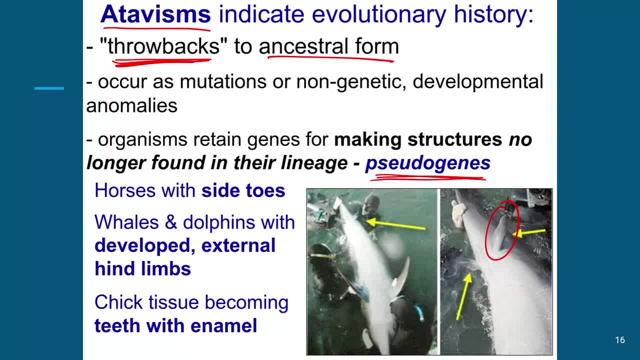 They've asked me not to, so I got too powerful. They were like he: he wants it too much, He's gonna be too good. So other examples: horses used to have a gene for more than one finger right. 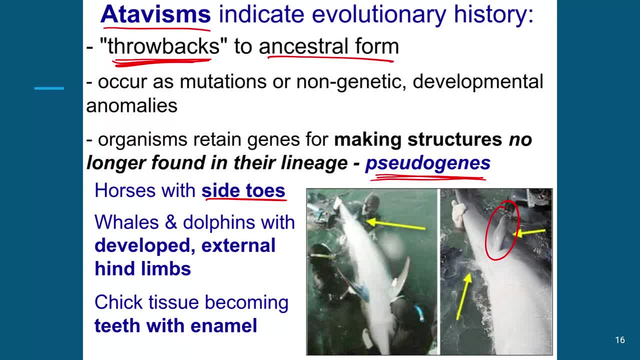 Cuz a horse leg is. just at the very end is just a finger, one big finger. Sometimes horses will have side toes. I've actually even seen pictures of cows with the same thing And it's just like a weird, like side. I don't, I don't really know. it almost looks like. 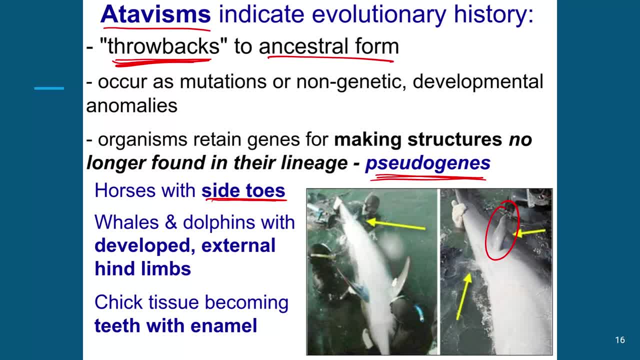 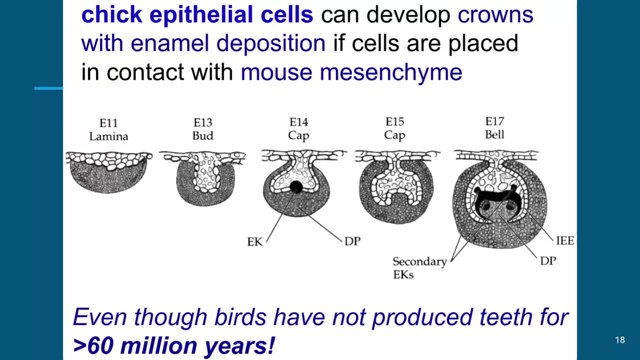 a claw. it's weird Dolphins and whales with external limbs, And then chick tissues have it chick having teeth, And that's what we'll look at. Oh, this was the baby with the tail Chick. so birds don't have teeth, right? 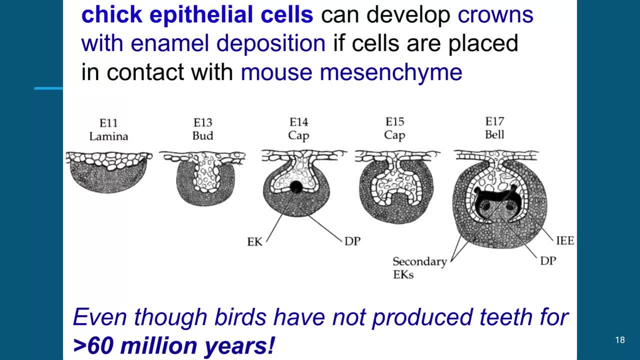 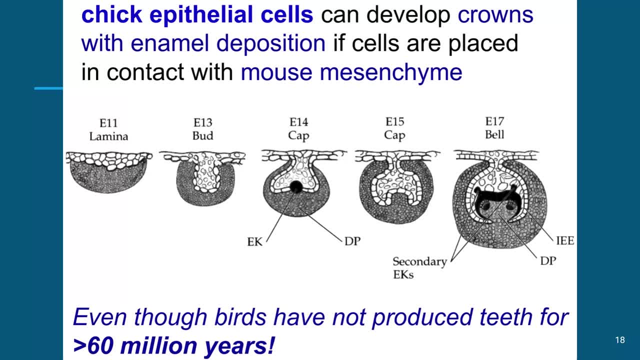 know, I saw like a tweet or something and somebody was like I can't believe it. I just learned that ducks have teeth. this is crazy. how did I not know ducks have teeth? And I was like I swear. on Friday we talked in class that birds don't have teeth. 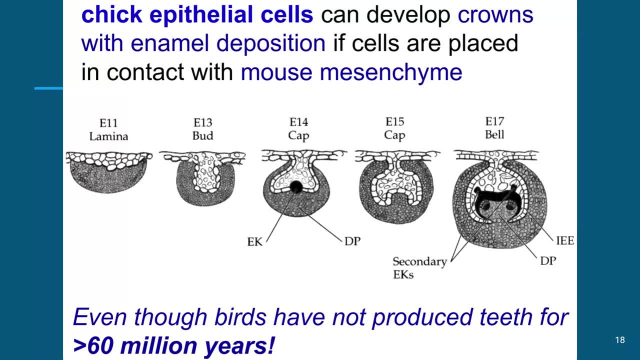 So I googled it. ducks don't have teeth. Somebody on Twitter is just an idiot Or just trying to get attention. They'll have like little ridges, right? If you've ever been bit by like a chicken or a duck or something. 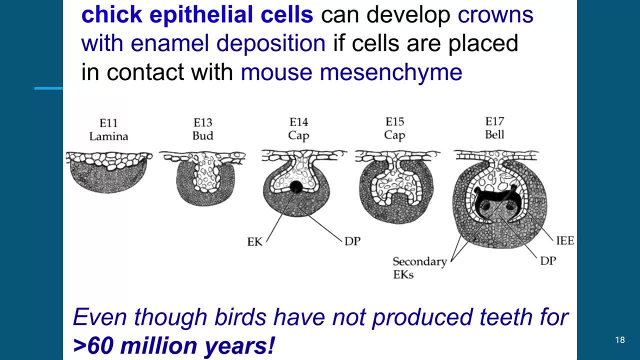 They have little ridges in their beak, but they're not teeth, they're just small protrusions of the beak itself And they're just. it's not like they chew with them or anything. they usually use them for like fighting or defense. 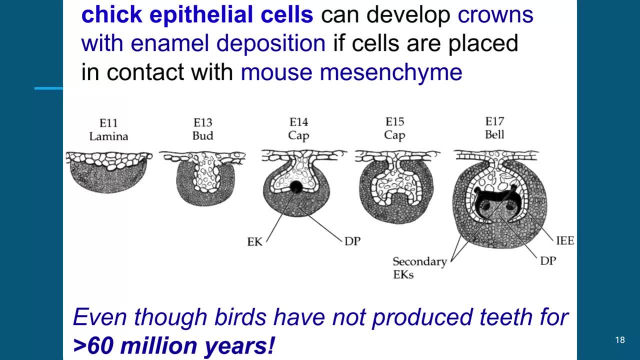 But they used to have a gene to grow teeth right, And this is kind of another way that we bridge the gap between birds and dinosaurs. Dinosaurs used to have- well, yeah, used to have- teeth, And birds, when they were kind of transitioning, had teeth. 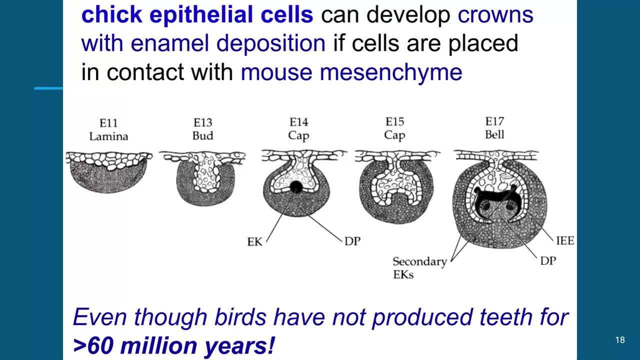 And they can do this. So they take mouse mesenchyme- I don't know what that is- And they put chick skin cells, basically mix it with this mouse mesenchyme, which contains genes to grow teeth. right, Because mouse mice have teeth. 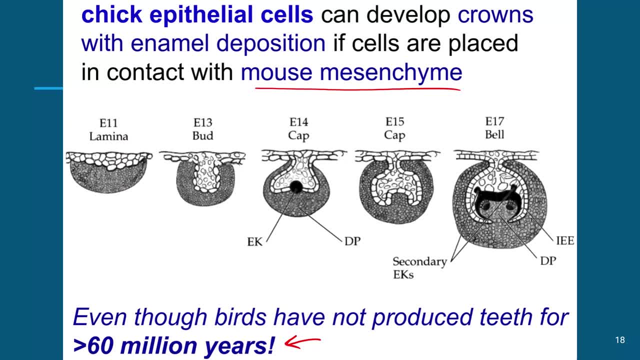 And so birds haven't had teeth for over 60 million years, including ducks. right, They can get chickens to grow teeth. I don't know what it looks like- I couldn't find any pictures- But I bet it's weird as crap. 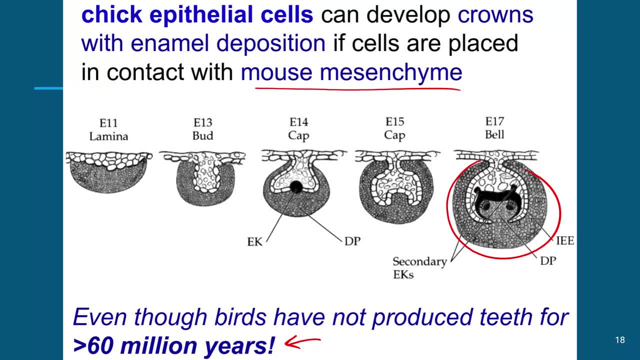 And they can get them to grow teeth. And it's again an example of an atavism. It's kind of a forced, derived, contrived atavism. But this gene is just waiting there. It's the mouse mesenchyme just happens to wake it up right. 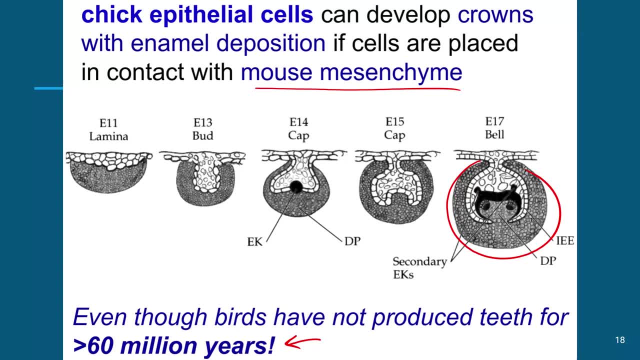 And now chickens grow teeth Kind of wild. I'd love to see it Because it would be weird. Um Yeah, Questions. So another example of an atavism. So you may see a question that said like if, and he'll change it so that it's not straight. 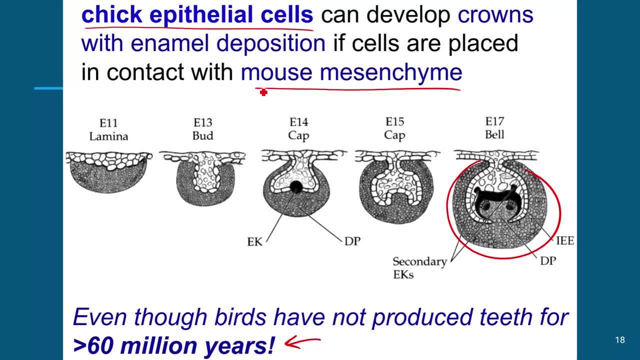 out of his slides. But you know, if chick epithelial cells were mixed with mouse mesenchyme and activated the gene for teeth, this would be considered an atavism, right? Because it woke up, if you want to think of it that way, an ancestral gene for teeth. 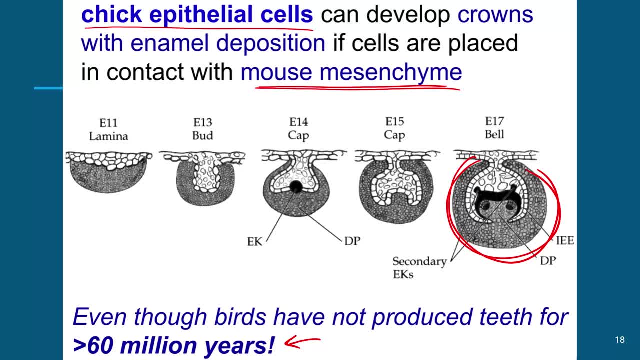 It's not that they mutated a mouse chicken And made mouse chickens with teeth right. They just used some enzymes or proteins or something in mouse genes to turn on chicken genes. Do you think you do like a true or false question with this? maybe you might change. 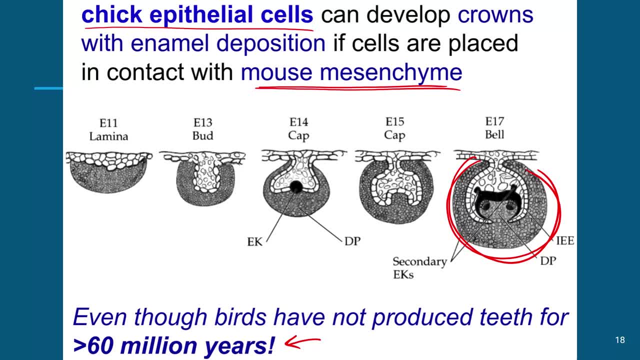 mesenchyme to something else. Um, That seems a little specific to me, Especially for him to just change mesenchyme to like I don't even know what else. That's probably too specific. But he could do a true, false question that would. it would give you an example of something. 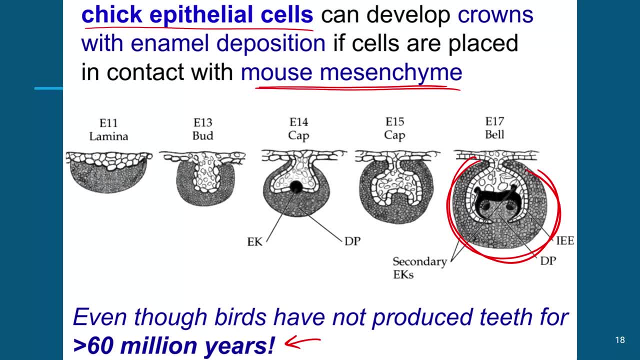 like this. Some scientist mixed this with that And they got this result. This is an atavism, True or false? And then you would have to deduce: did they cross breed something and get a mutation out of it? Did they change its genome? 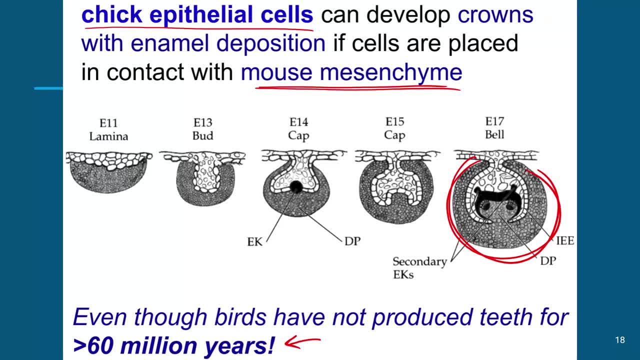 Or did they just use a few chemicals, Chemicals and interactions and things like that to turn on an old gene? So yeah, You could see a true or false, Probably just not that specific. It would be a bit of a douchey move. 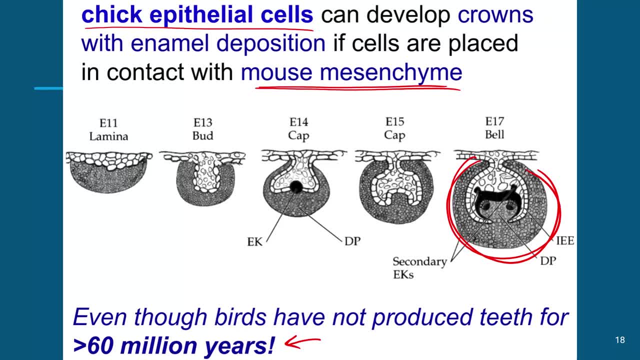 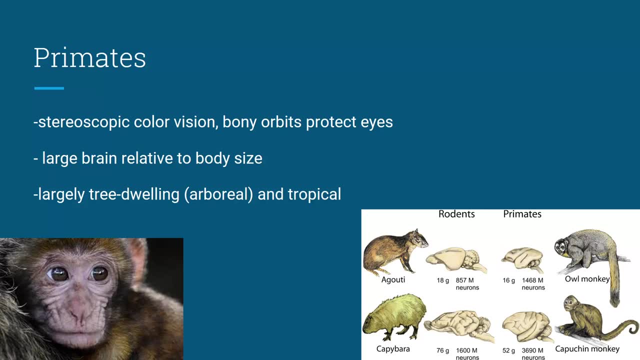 But it depends on how Dr Messina is feeling, right before he makes the test right. Other questions: We've got like 10 minutes left, So we're going to breeze through. human evolution Starts with primates, right? So first off, important things to know about primates. 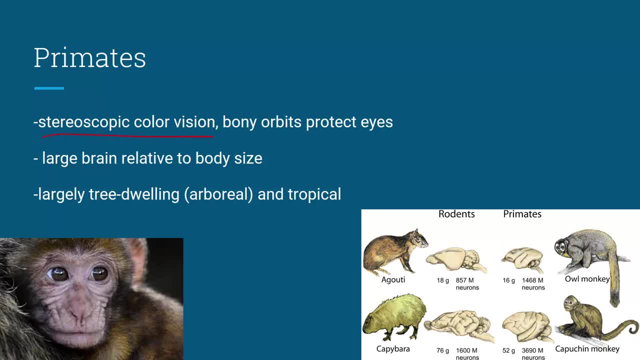 They have stereoscopy. They have stereoscopic color vision. They have two eyes facing forward And they can see trichromatic right- the three primary colors, And they have bony orbits around their eyes, which is essentially the eyebrows and this 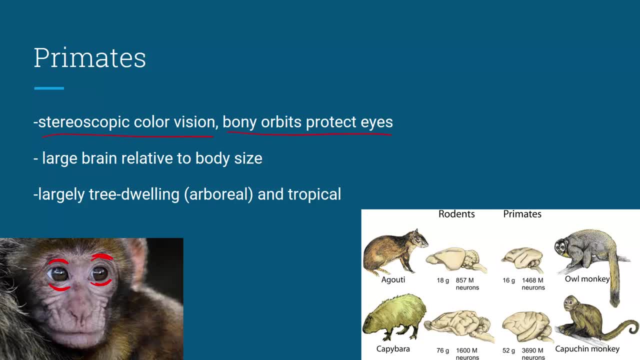 like under your eye that you can feel it if you go like this. right, unless you have a sinus infection, Don't go like this, It hurts a lot Again. large brain to body size ratio Ratio. They mostly are arboreal or tree dwelling and tropical right. 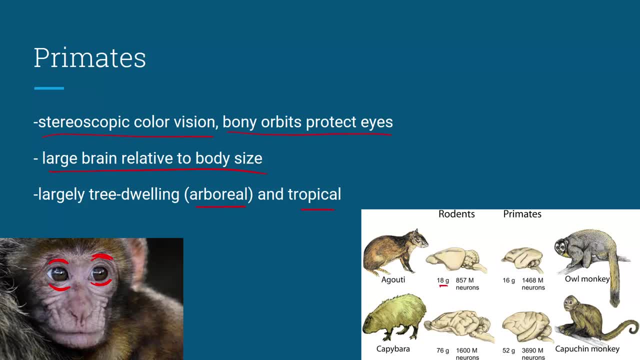 So this is just kind of an interesting comparison. And a agouti has an 18 gram brain with 857 million neurons. An owl monkey has a slightly smaller brain at 16 grams, but has almost twice as many neurons. right, So their brain isn't per se larger, but it's denser. 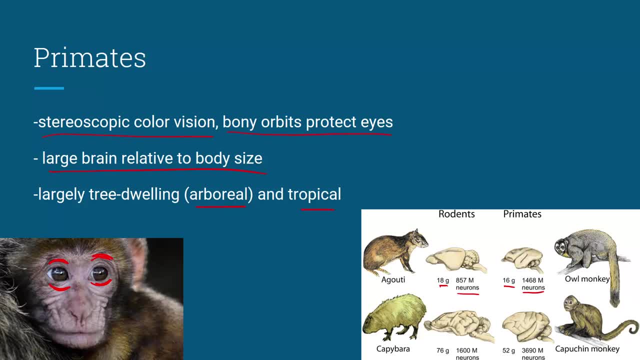 And it's more complex, Right? Yes, The folding in the brain is what allows it. It increases surface area without necessarily increasing volume or mass. So the human brain isn't even the biggest brain out there, right? Whales have larger brains than we do. 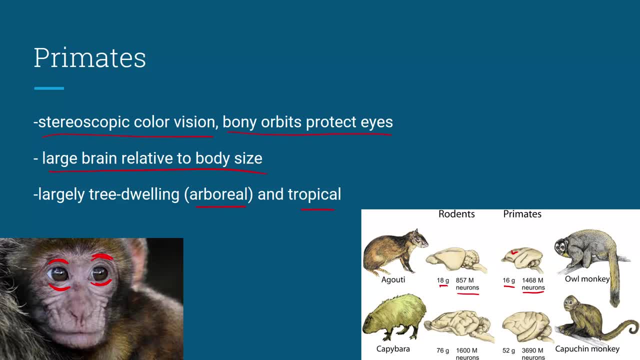 A lot of animals have bigger brains. Brain size doesn't equal intelligence, right? So don't get that confused. When we say large brain to body size ratio, Right, We're not saying they have really big brains, right? An owl monkey has a smaller brain, but their brain to body size ratio they have a much. 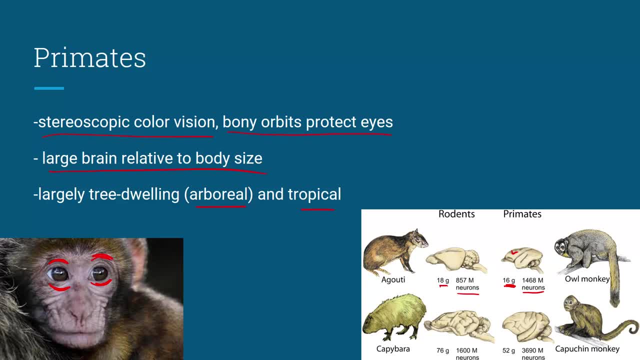 larger brain for how big their body is. But again, that's not what makes them smarter, It's the neurons that they have and the folding that they have right. So they weighed Einstein's brain after he died And it was actually a couple grams below average- his weight of his brain. 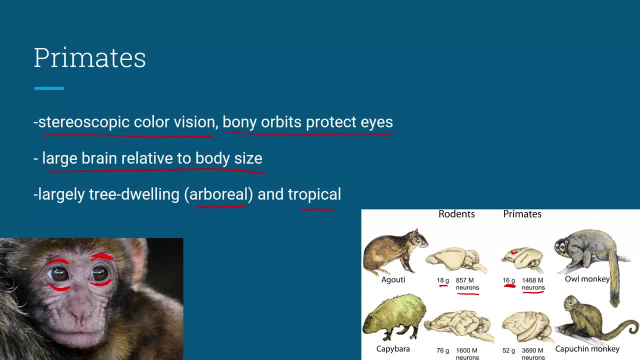 Because it doesn't matter how heavy, how big your brain is. But they saw an abnormal amount of folding in his brain So it had a higher surface area, Right. So he cheated. He's not actually like better than anyone, He just had a foldy brain, a creakly brain. 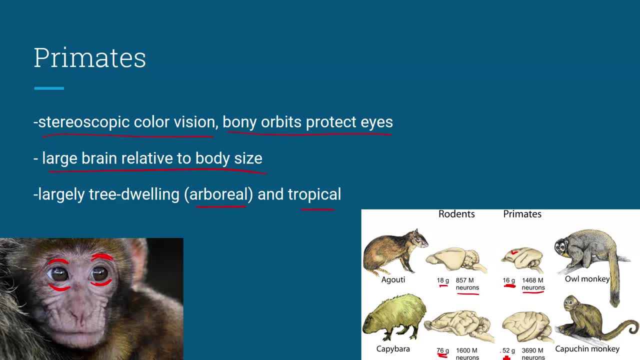 Right. And again you can just see that 76 gram brain, 52 gram brain, but twice as many neurons Right, Over twice as many neurons Right. So this is part of what makes primates some of the more intelligent species on the planet. 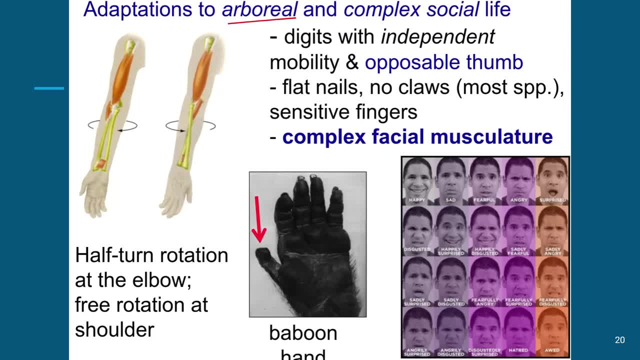 How they adapted to become arboreal was partly that they can turn their arms at their elbows just like we can. Right, We're technically primates And they have free rotation at the shoulder, meaning they can do these kinds of motions Right. 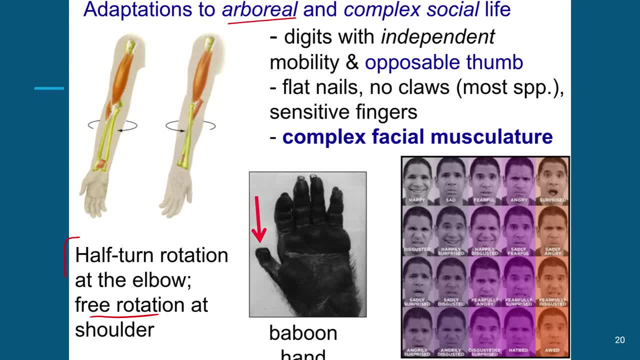 So it's very handy when you're swinging through trees to be able to turn your arm and to be able to swing your shoulder Right- The opposable thumb. quite an advancement for humans. Right Comes in handy. They usually don't have claws. 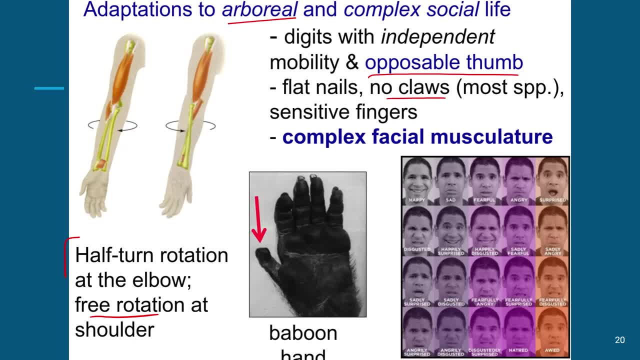 Right, Because they're not climbers in the sense of digging their claws into things and they're not fighters in the sense of using their claws. So they usually use them more just for grip Right And they have very sensitive fingers, quite handy for when you're going from vine to vine. 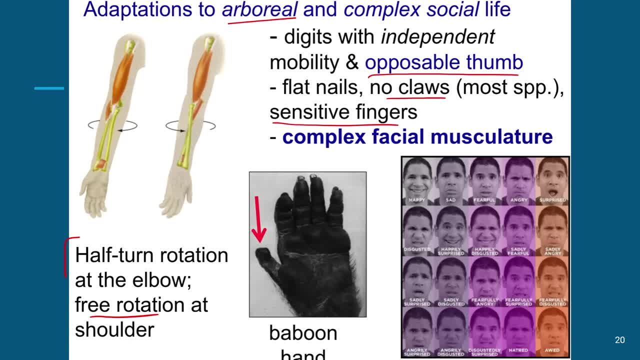 You want to be able to feel them, Right. So they have very, very sensitive fingers. We have very, very sensitive fingers, And something that makes them able to have very complex social lives is facial musculature. Right, We have very complex musculature in our faces compared to most other animals. 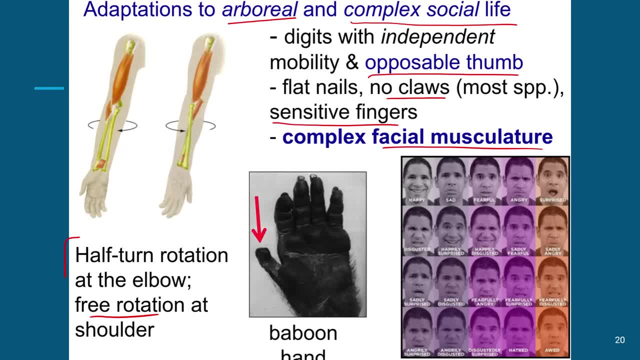 Right, So this is why- chimpanzees and orangs and all those and us, We can have really complex social lives and structures. We're able to physically display more emotion. Therefore, we can interact more fully. Right, It really just boiled down to: we have more muscles in our face, we can express more emotions. 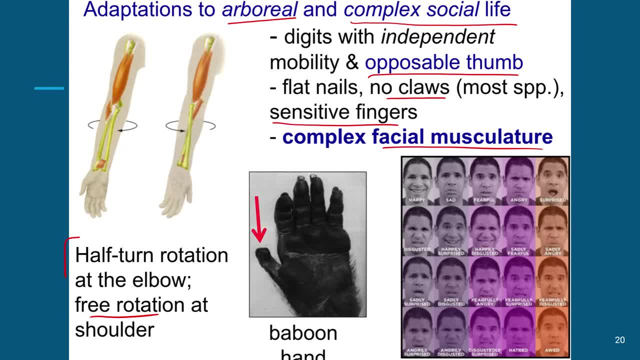 Right, I should have put it in here. I have a video of a magician doing a card trick- I think it was with a chimpanzee- And he just makes a card disappear Like kind of standard magic. And you see the monkey like raise his eyebrows and his eyes get big and his jaw drops and 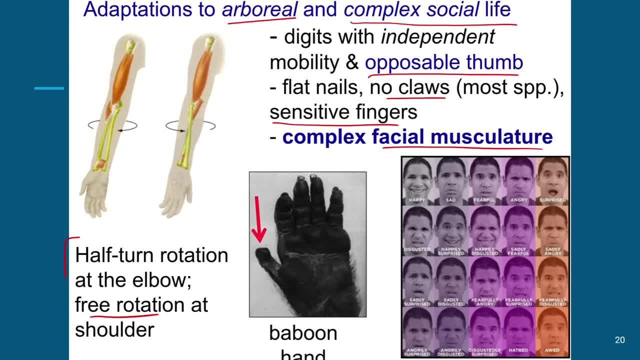 he goes and he, like, puts his hand on the glass and he's trying to figure it out where it is Right. Primates can display emotion in a way that most animals can't. Right, You probably think that your dog's all cute and he can smile and he can look at you. 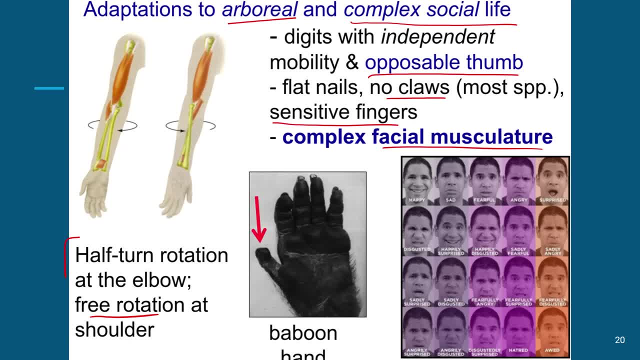 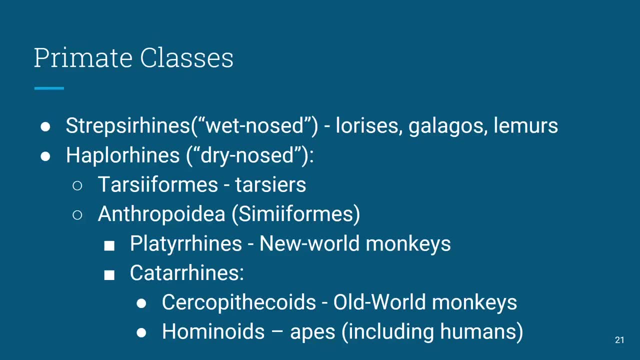 That's about it, Right? Your dog can't laugh. Your dog can't look surprised. Sometimes they can, But they don't make as many facial expressions as us, Right? They don't have that same musculature. Okay, I'm going to pick up the pace here, because we've got to get through it. 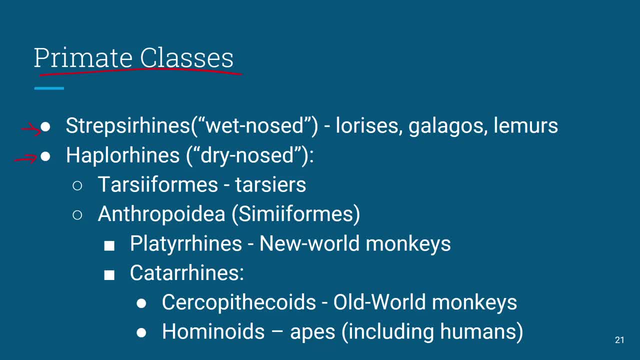 So primate classes break down into two names: Strepsirhines, which means wet nose, So these are things like lorises, galagos, lemurs. I don't know what those first two are, I just know how to say them. 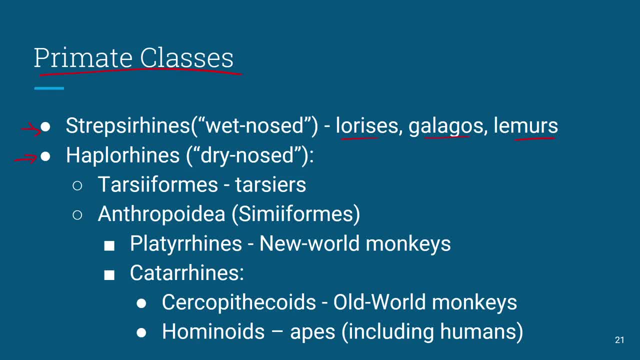 And then everybody knows what lemurs are, Right. You guys watch the boom-a-foom, right? A few of you know what I'm talking about. What's the other one? I'm thinking of Madagascar Lemurs, Right? 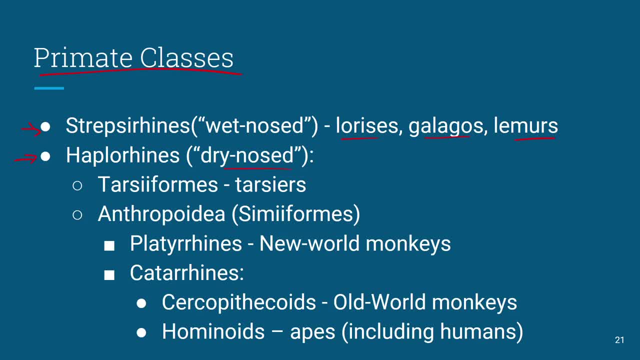 Then you have the haplorhines- means dry nose, Right, And it's literally because their nose isn't wet like the strepsirhines. So you have your tarsiformes, which are tarsiers. They got real creative on that one. 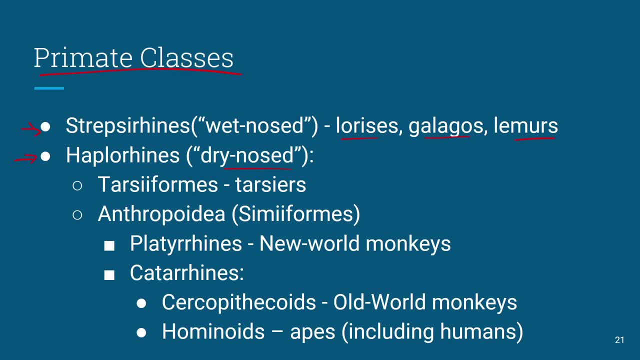 Not really anything important to talk about there. Tarsiers are tarsiformes, That's it. But then the other breakdown inside of the haplorhines- still the haplorhines- is that they're not wet. They're not wet. 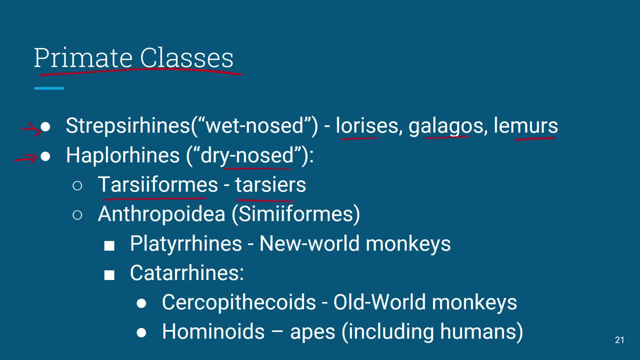 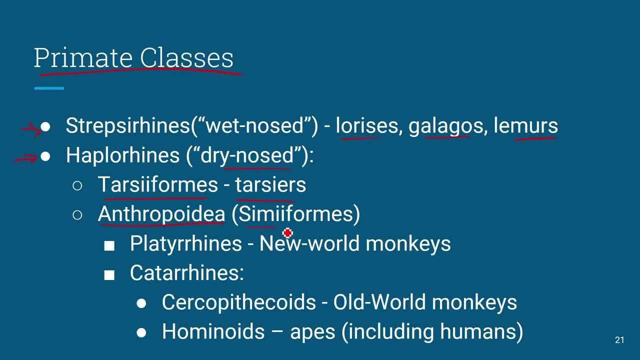 So the ones you would find in the New World as in like South America. And then you have old world monkeys or circopythocoids inside the catterynes. Those are a new world rabbit bumblebee that comes together. Those are hunter-g fantasies. 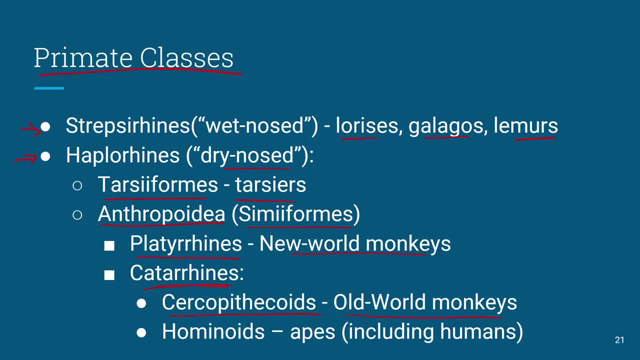 But they're not tarsiers and will not ever like. you can all tell that, Right. Yeah, and also inside the catarines, hominoids or apes, including humans. You do have to know all of these names. 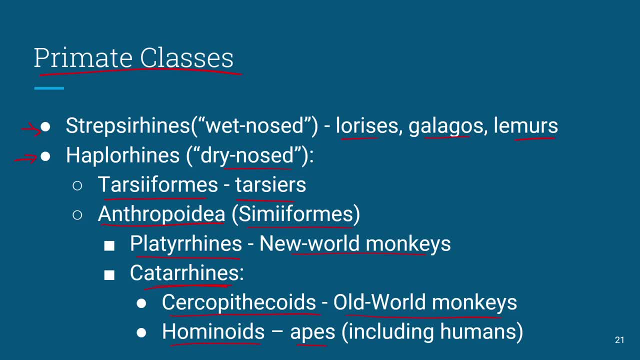 You do have to know the order, So you have to know it's strepsirines and haplorines, but then haplorines breaks into tarsiformes and anthropoids, and anthropoids breaks into platerines and catarines. 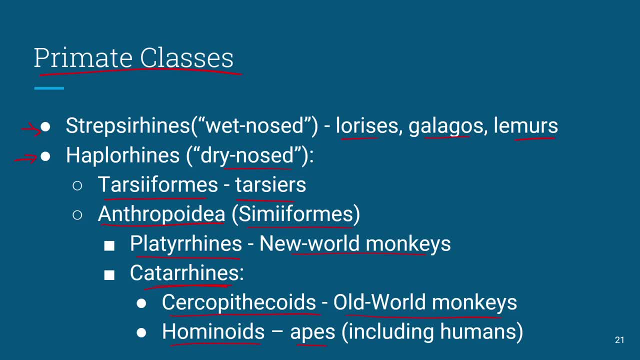 and then catarines into circopithicoids and hominoids. You do have to know that. I would also know that strepsirine is wet nose, haplorines dry nose. I would know platerines are new world. 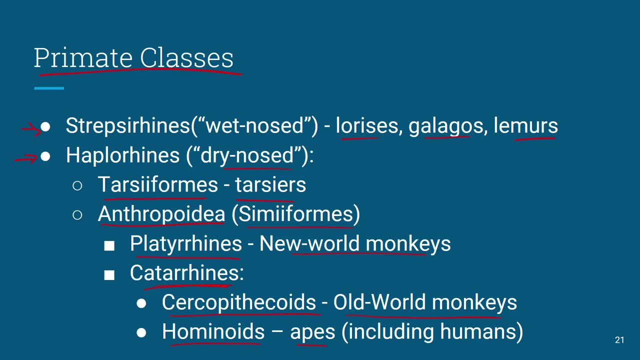 and circopithicoids inside the catarines are old world. Tarsiers wouldn't be that hard to remember And then maybe just know anthropoids and simiformes are the same thing. Yeah, So what does it just mean by old world? 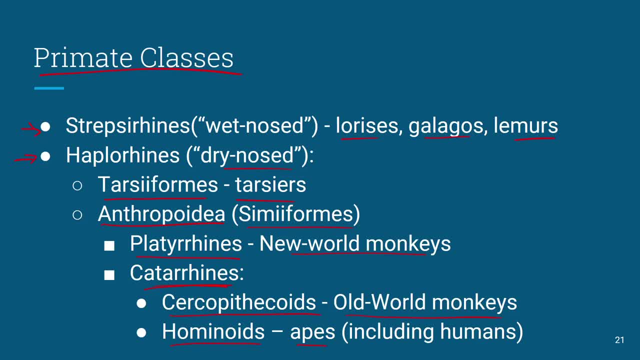 Africa. So chimpanzees, Chimpanzees, orangs, gorillas and any kind of monkey that you would find in Africa, Not monkey, ape that you would find in Africa, But again, and I guess, so I guess I said it a little bit wrong. 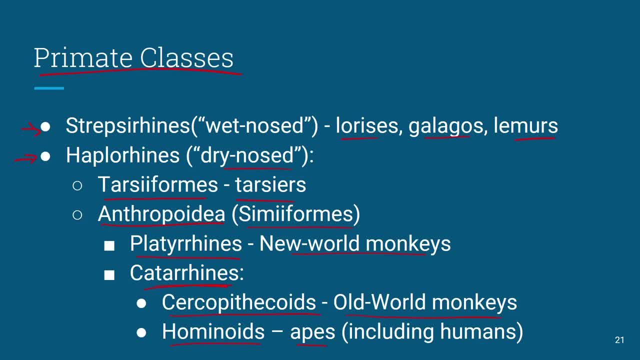 Old world monkeys means African monkeys and then separately is apes, So chimpanzees and gorillas and all that are hominoids. Circopithicoids are like baboons and that big problem. It's like a little hibiscus monkey that had like the huge nose. 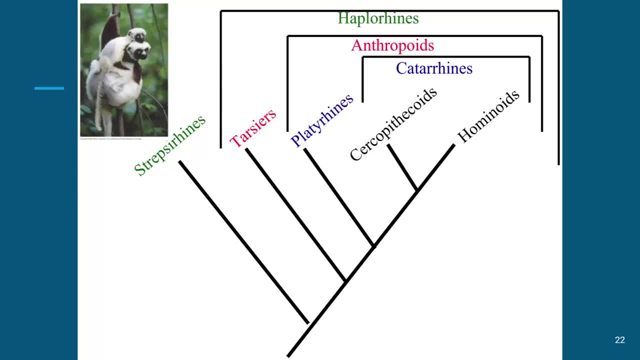 if you guys remember that from class. But we'll look at that. We'll get into each of these. So this is how they break down, right. Strepsirines broke off and are their own species, Then evolve or not evolving from, but sharing ancestry. 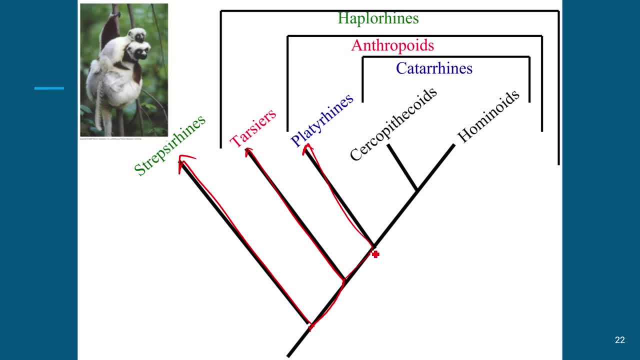 You have the tarsiers that break off, then the platerines, then the circopithicoids, all the way up to the hominoids, And then you can see how each one falls under a category. You do have to know like strepsirines are separate. 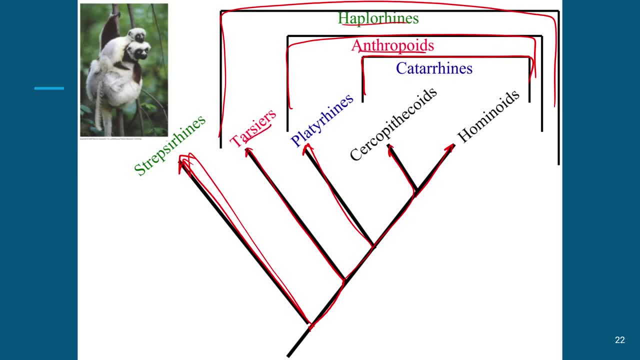 from haplirines. Tarsiers are not part of the anthropoids. Platerines aren't part of catarines, right? So essentially you have to know the name of each and how they branch from each other. So I would spend a lot of time with this. 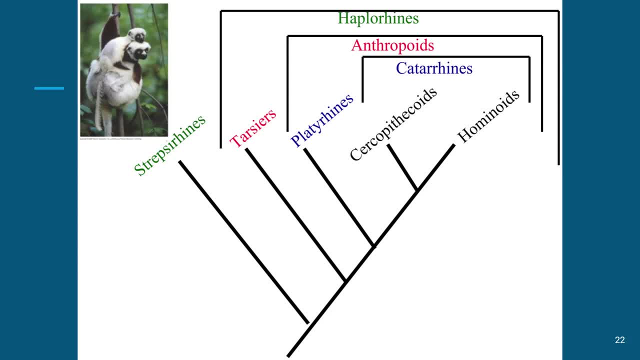 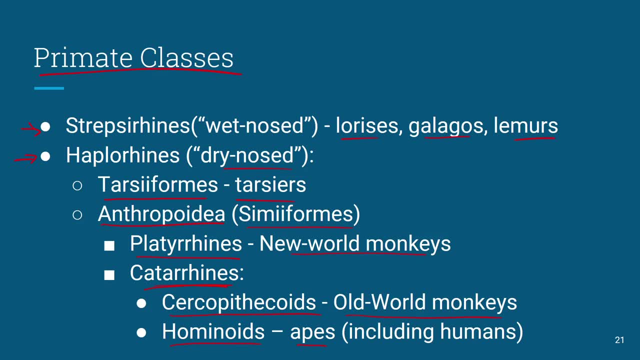 I remember I think I got a question. I think I remember a question about whether platerines or circopithicoids were New World monkeys, And I think I also got a question on something about strepsirines versus haplirines. 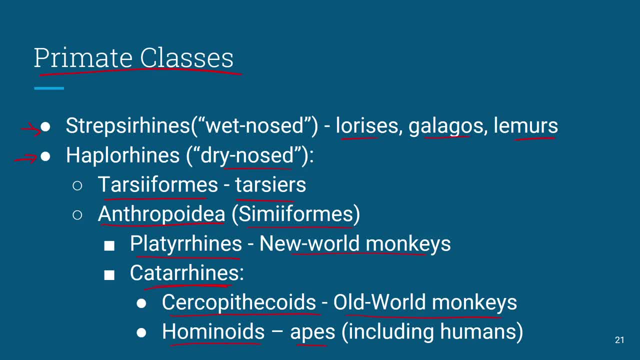 I'm not saying that's what you're going to see. I'm just trying to tell you there were, at least as far as I remember, at least two questions essentially just off this slide, right. So this is important stuff to know. 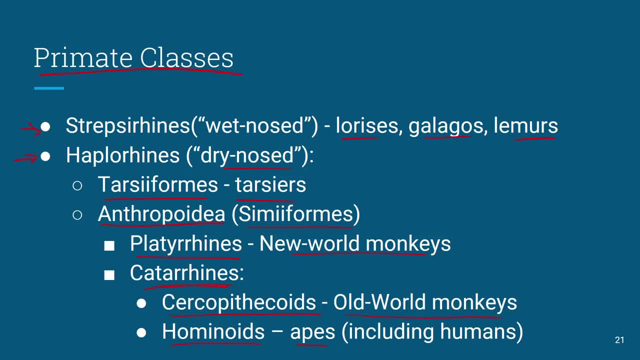 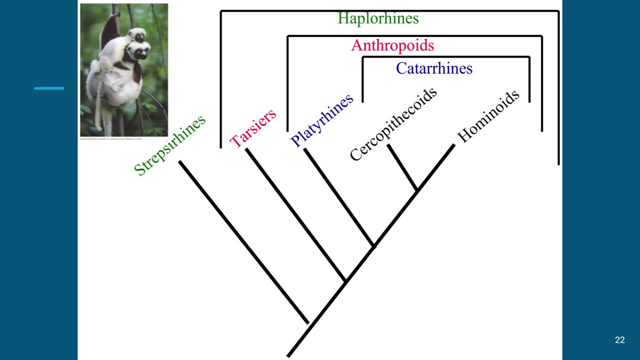 It's not hard. You do have to take the time to memorize it, right? So, again, this is something that I would start drawing it, I would start writing it out, I would start making charts or graphs, or even just make your own phylogenetic tree. 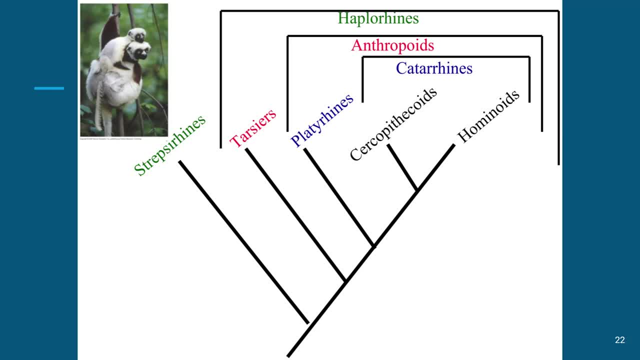 but do it over and over and over. So when test time comes you're not going. how did it? you know, you remember, you can maybe even draw it yourself, right? So the anthropoids, so remember, the anthropoids is all of these. 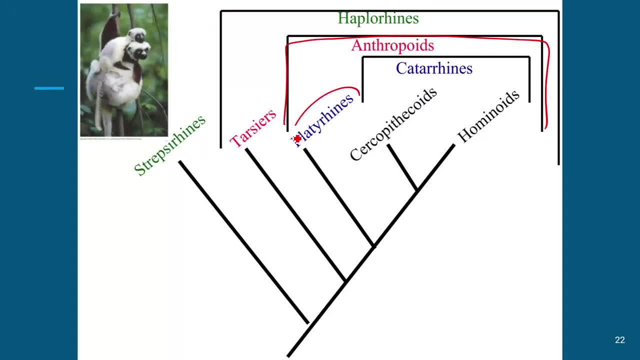 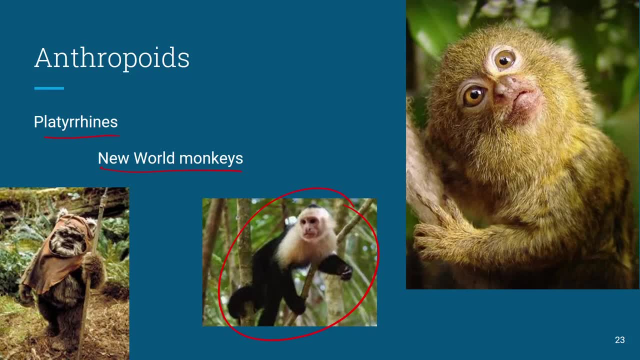 You have first the platerines, right? So we'll look at platerines. first is the New World monkeys, right? So the capuchin, the. I don't know what this is, but then it made me think of an Ewok. 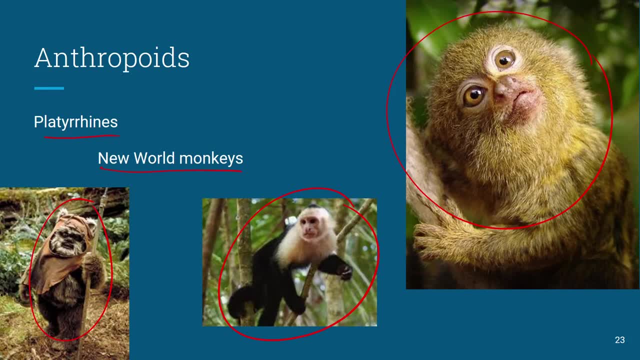 I don't even know why I was like this kind of looks like an Ewok. Ewoks are not New World monkeys, They're fictional creatures from Star Wars. So New World monkeys- anything you would find in South America, right? 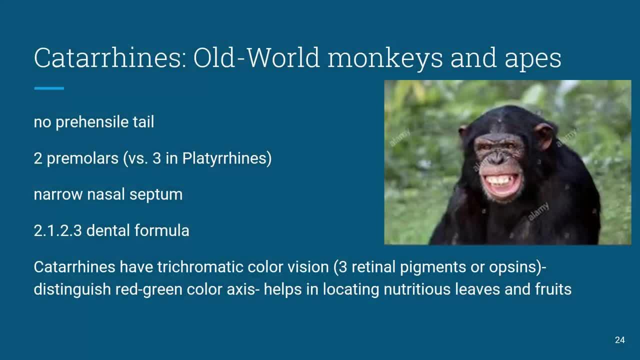 Or Central America, or Mexico or the Bronx Zoo. Yeah, that's all we need for those Caterines. have the Old World monkeys and apes, right? So cercopithecoids and hominoids? They don't have a prehensile tail. 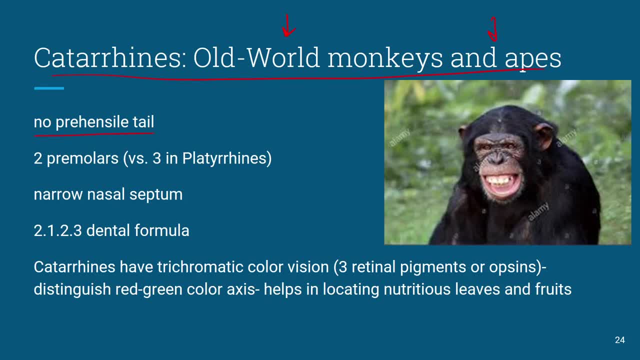 What does prehensile mean? They can use it like a hand. yeah, So Old World- or sorry, New World, monkeys can use their tail almost like a fifth limb. right, I, actually I held hands with a spider monkey once. 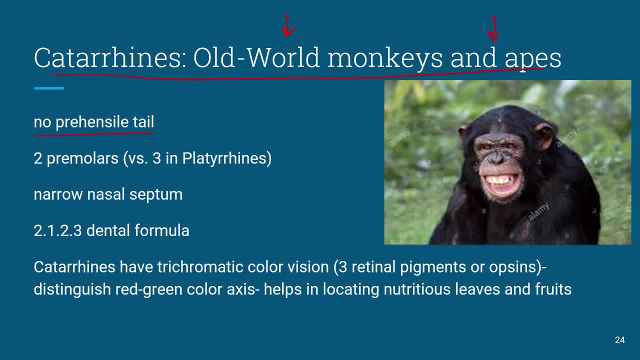 and they have like really weird long fangs on their fingers. but then he like wrapped his tail around my wrist and it felt like he was grabbing me. They have muscles in it that allow them to physically grab things. I think in fact. oh, I thought yeah. 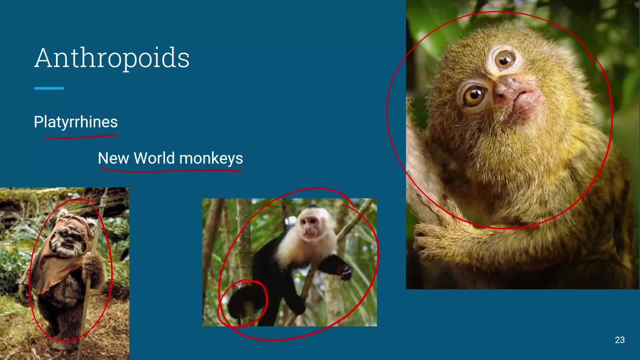 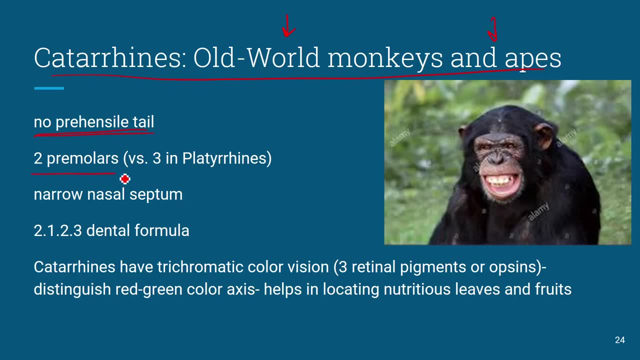 They'll grab onto trees and vines and whatever with their tail right. So that's a prehensile tail. Caterines don't have that. okay, They have two premolars rather than three. Platerines will have three premolars. 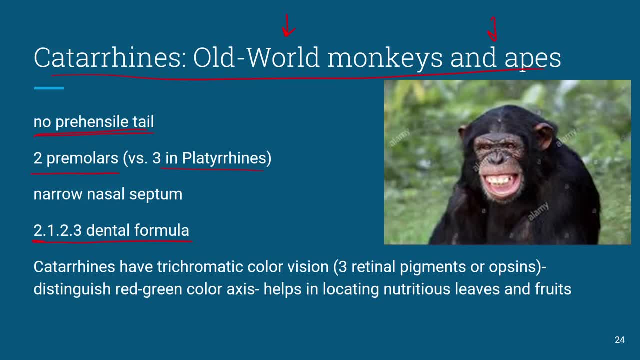 Which comes to this dental formula, This is two incisors right And we have the same. so if you have a hard time remembering, but you know your own teeth well enough, you have two incisors right: Your front teeth and the teeth right next to them. 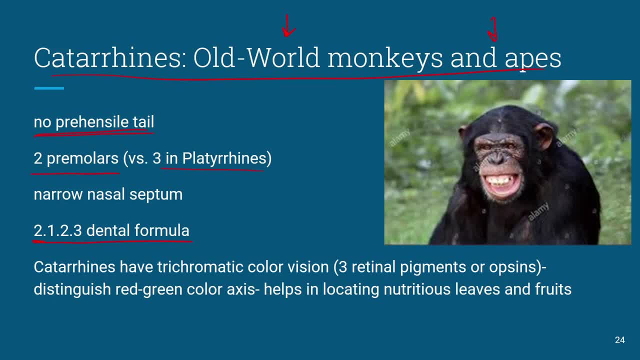 So really four, but you split it in half and you just look at one side. So you have your two incisors right Front teeth and the teeth next to it. You have one canine, two premolars. You can even kind of feel them with your tongue. 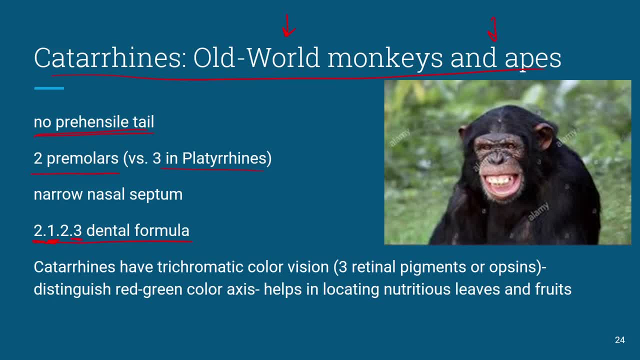 They're the pointy ones before your molars, And then you have three, Three molars, right, But the platerines have a two, one, three, three. I think You won't be tested on that. You could be tested on that though. 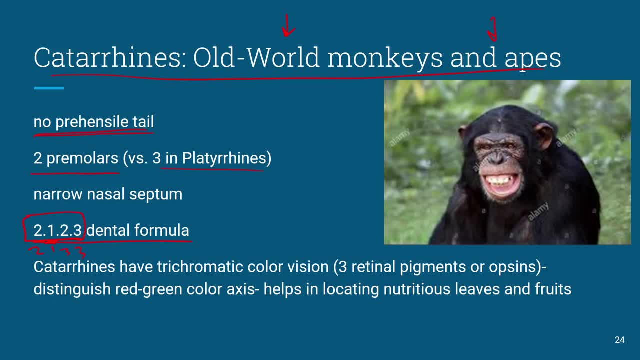 Two, one, two, three: Is wisdom teeth counting as the third? I don't know. I'm trying to feel it with my tongue, Probably Yeah, I would say. yes, I don't know, try and feel it. I'm like I don't have wisdom teeth anymore. 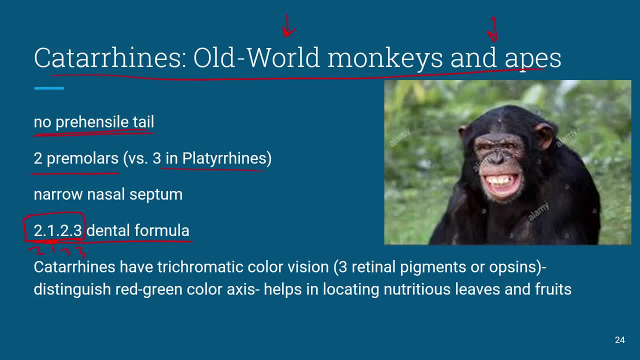 but I'm pretty sure I'm running my tongue, I don't know. So catarines have trichromatic color vision. They can see the three primary colors in the mix they're in And that just helps them find food better, right. 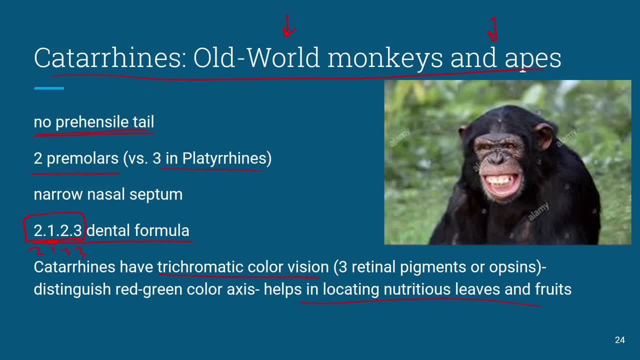 Make sense. So I would know they don't have a pretensile tail. They have the two rather than the three premolars for a two, one, two, three Dental formula. again, that's just starting in the middle of the mouth and going this way. 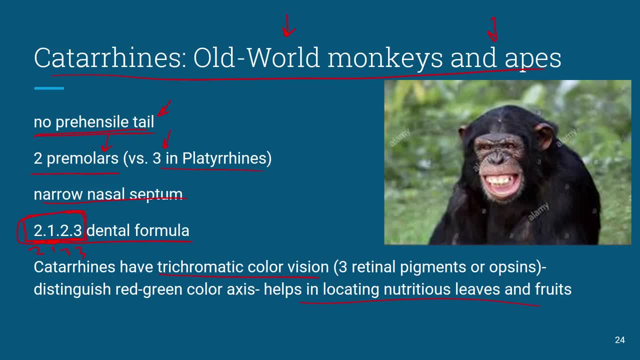 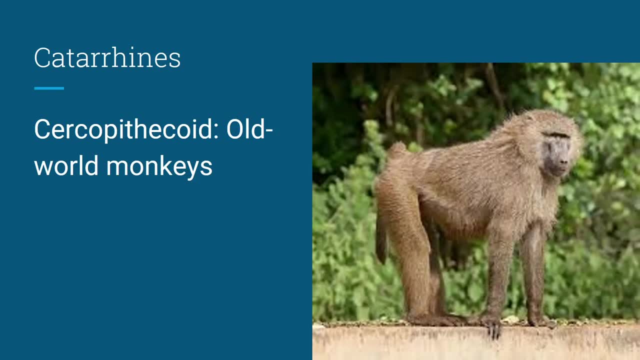 They have the nasal septum very narrow and they have trichromatic color vision. So old-world monkeys would be the circopithecoids. like a baboon, Notice he has a tail right. It's just not prehensile. 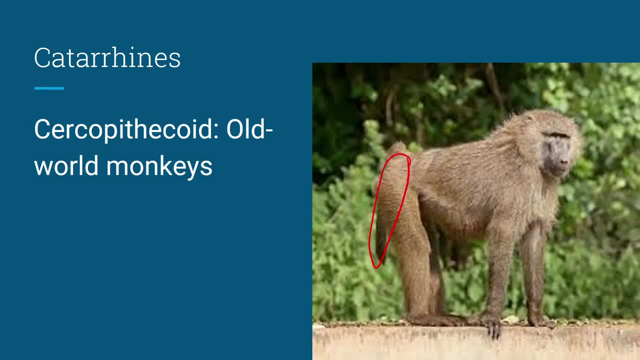 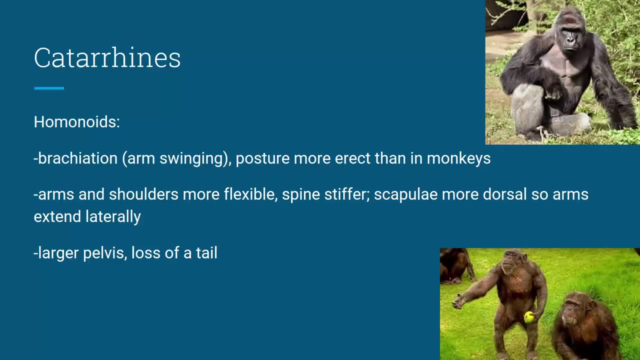 It doesn't grip, It doesn't have the muscles in it. So baboons don't use their tails to grab onto trees and things, They just use them for balance right. Then you get into the hominoids, So they have arm swinging. 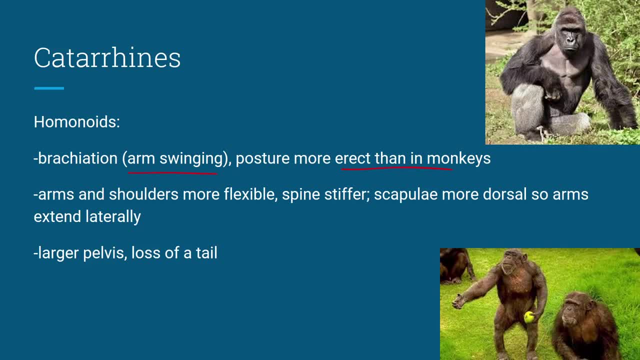 They're more erect right. So, apes, you know they can sit up right. Does anybody know who this is? That's Harambe. I googled gorilla and he was the first picture that came up And I was like, oh, it's Harambe. 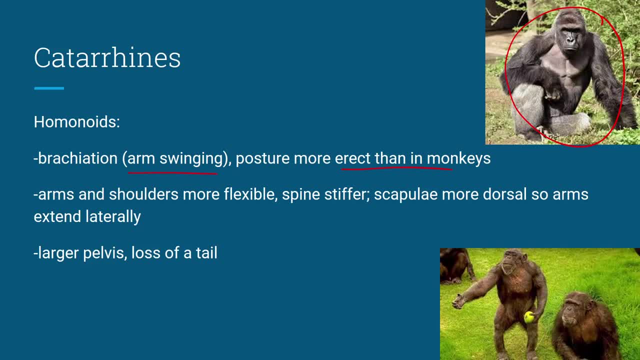 I remember him. He was big in like 2010 or whatever that happened, So they're big. So they're big. Their arms and shoulders are more flexible. Again, this is just because of the way that their skeleton is set up. 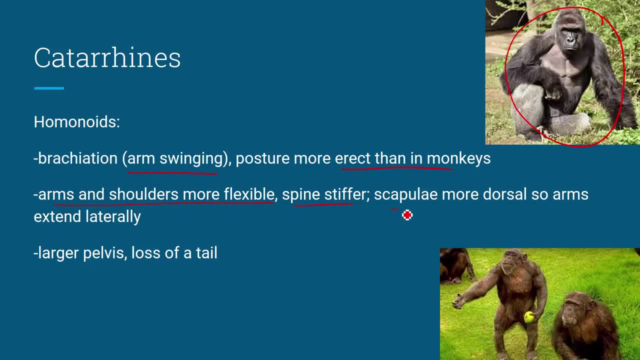 They have a stiffer, straighter spine. Their scapula are more dorsal right, which just means that their arms can stick out more sideways right. Apes can bend their arms back like this, Other monkeys can't. They have a bigger pelvis right. 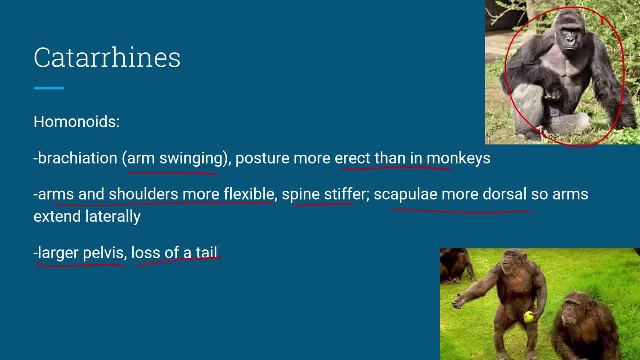 part of which allows them to stand on two legs, And they don't have a tail at all. right, So think of, like chimpanzees and gorillas, or humans, No tail. This is the list that I would use to make my chart.